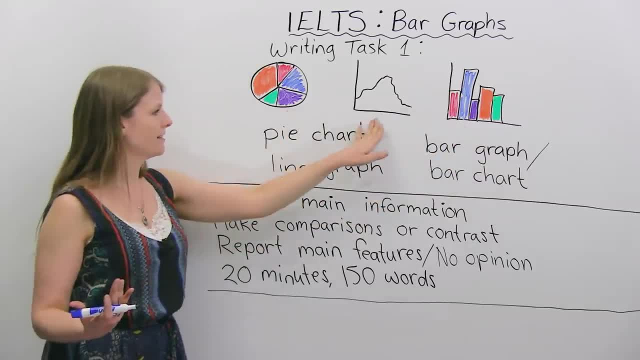 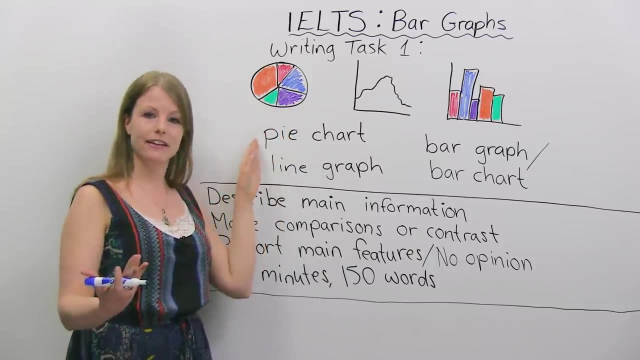 of charts or graphs. We have this one, this one and this one. This is called a pie chart. Okay, I've covered this in another video, so if you're interested in learning how to write about pie charts, you can check out that video. 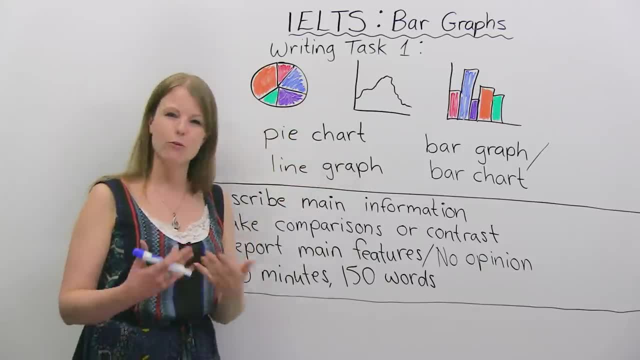 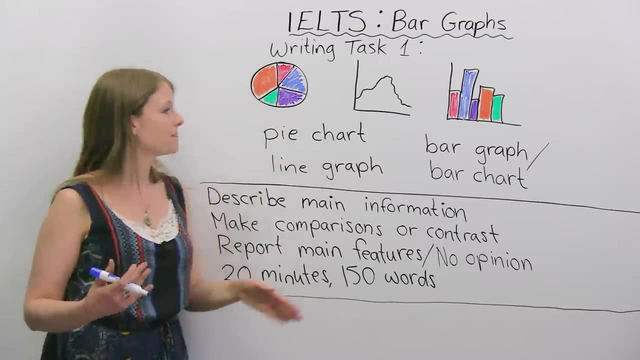 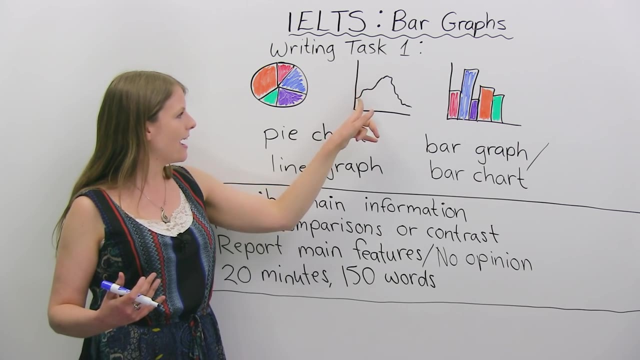 But you'll notice, with a pie chart it looks kind of like a pizza or a pie. It's in a circle and it's It has different colors representing different percents. We have here This is called a line graph, So you'll notice that there's a line and 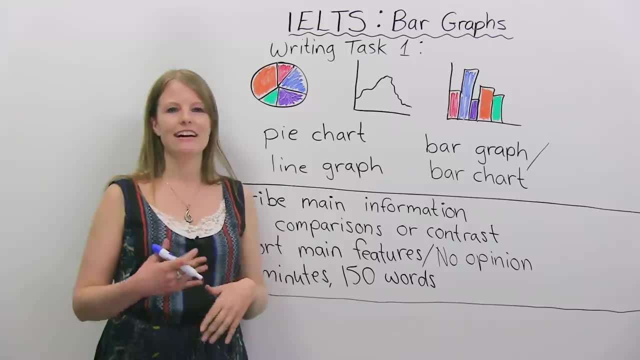 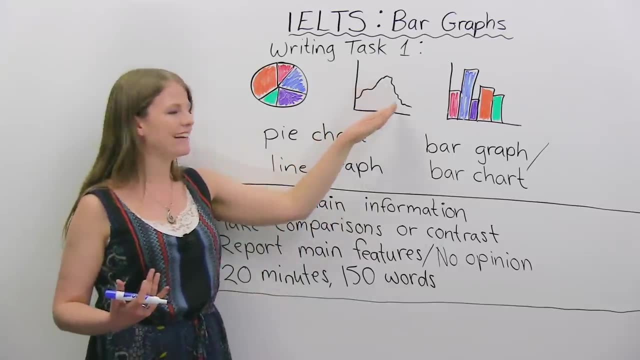 you know, sometimes this represents time, sometimes it represents other things, but with a line graph you'll notice, like you know, increases and decreases, but it's one connected line. We're not covering either of these in this video. What we're going to. 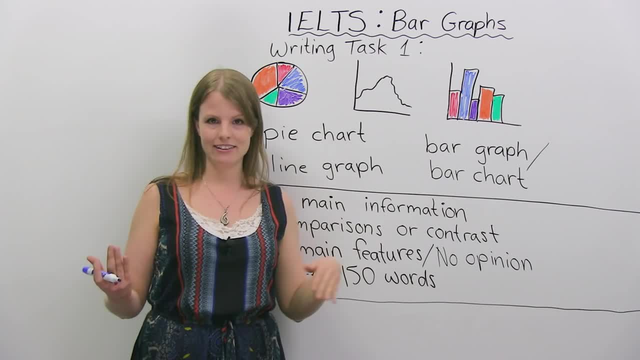 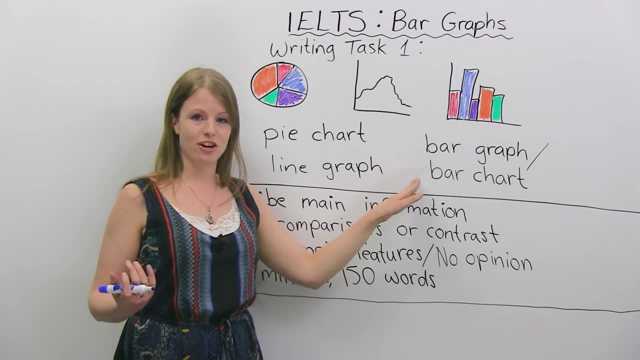 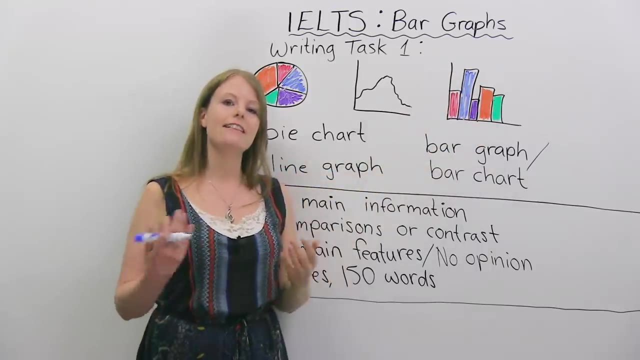 be covering is Another thing you might see on the IELTS, which is you might be given a picture like this. This is called a bar graph or a bar chart, So we have here these rectangular-shaped things that are each a different color. These are known as bars. Okay, So I know a bar is. 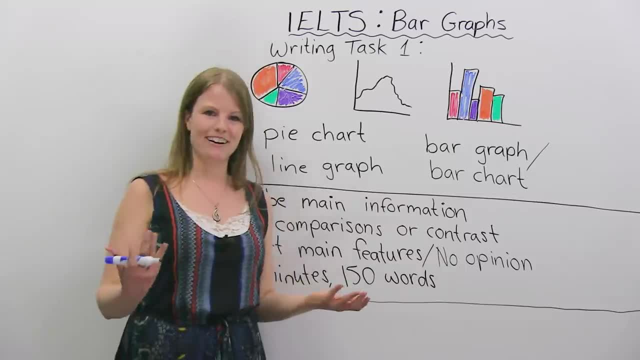 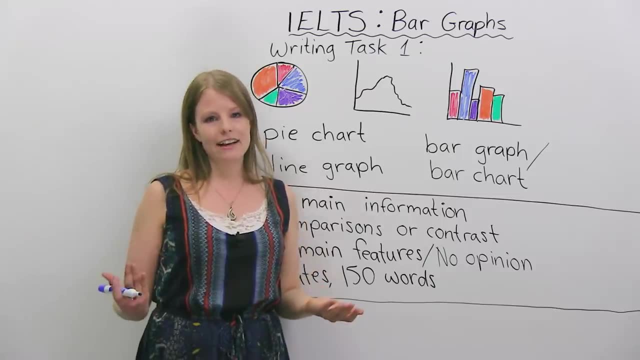 a place you go to buy beer, but in this case a bar, is not that, It's actually this kind of rectangle on the chart. Okay, So on the IELTS, you may get a picture of something like this. You might actually get a picture. 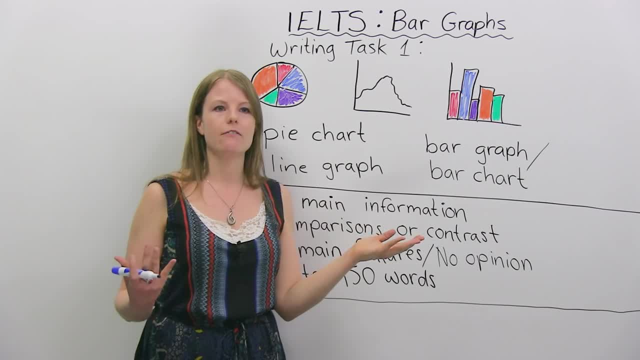 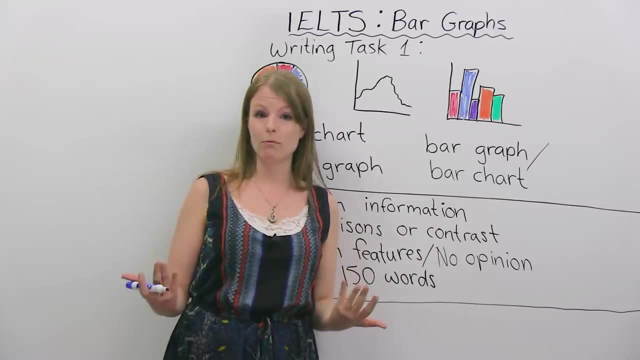 of two things together, or you might get a picture of something a lot more complicated than this. In this case, we're going to talk about what would you do and say and what are some tips if you get a picture of a bar graph or a bar chart. 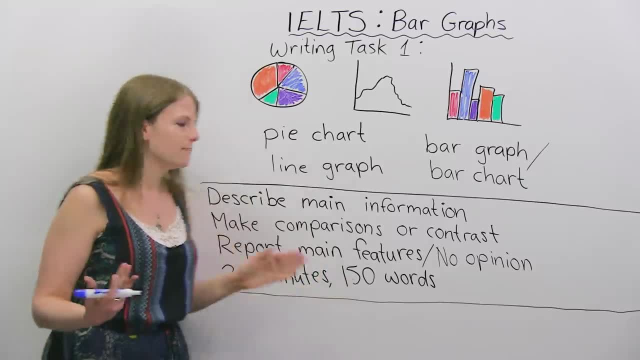 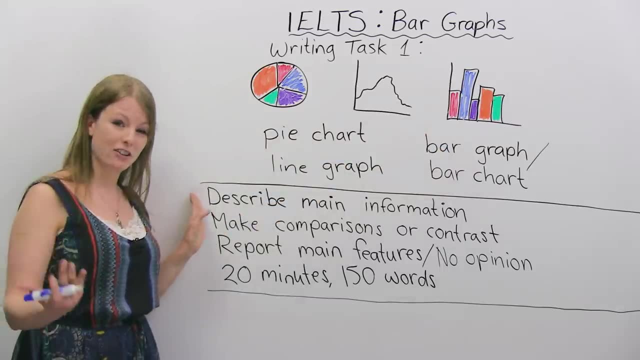 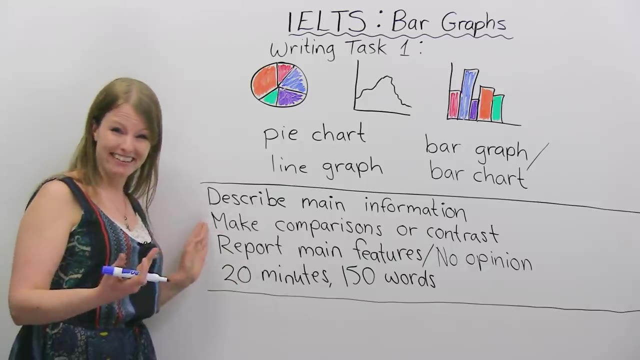 Okay, so what are you going to have to do Specifically? they're going to ask you, after you get a picture like this, they're going to ask you to describe what you see. Okay, So you're describing the main information. You're also going to have to maybe make comparisons. 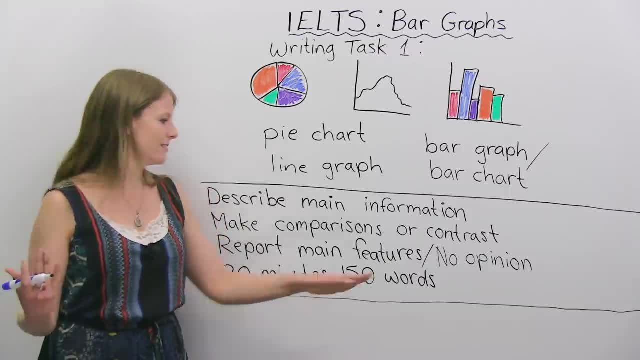 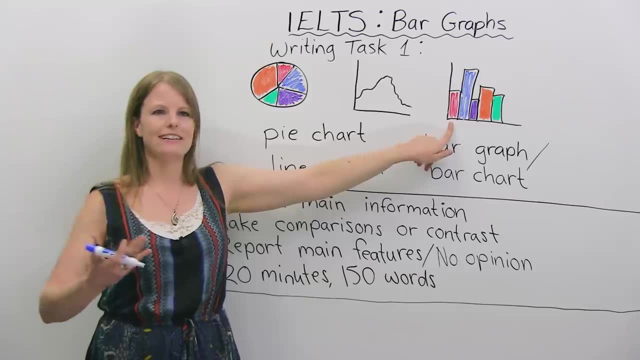 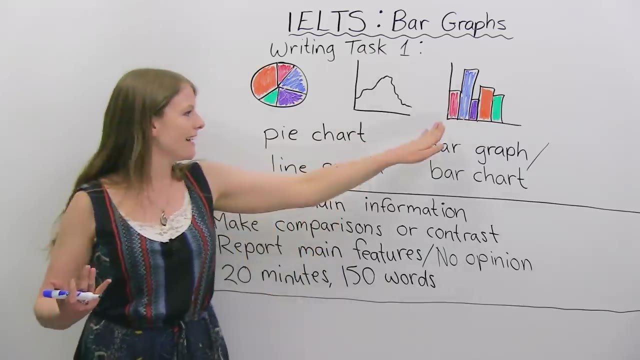 say how things are similar or how things are different, which is contrast. So, for example, if this is, you know different activities, maybe you might say that the red is shopping and the blue is golfing. In this case, shopping is less popular than golfing. Okay, 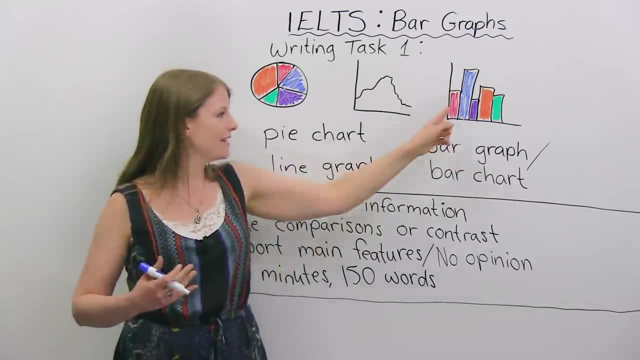 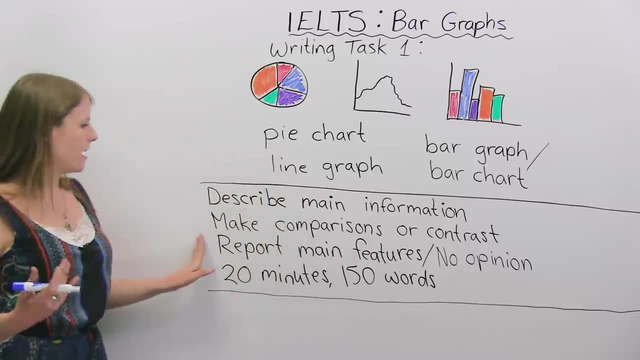 So pretty much you need to compare the different bars and say what are the same about them, which ones are similar and which ones are different. You're also going to have to report any main features or trends. Okay, So maybe you'll. 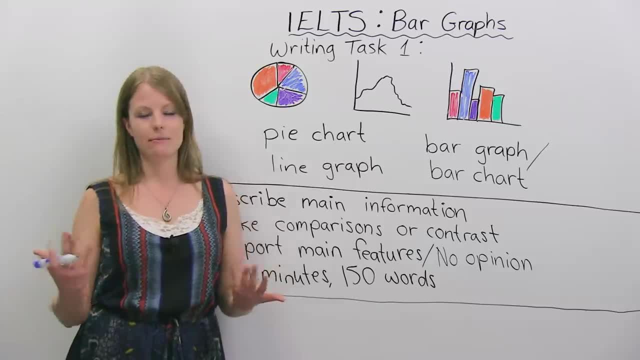 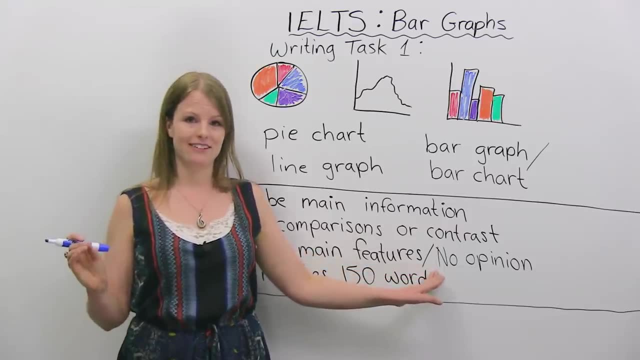 see a pattern and you're going to have to write about, you know, some of these main points. you see, when you look at the visualization, You do not write your opinion, Okay. So if this is a graph on education, maybe this is. 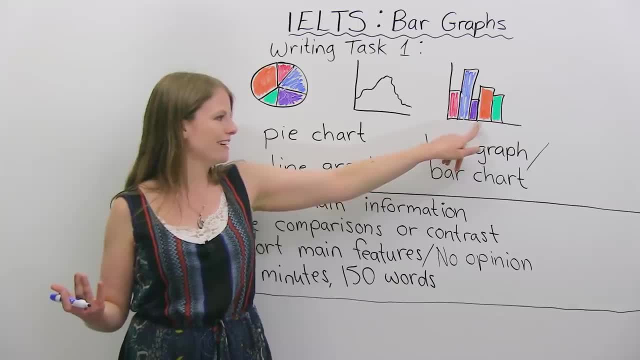 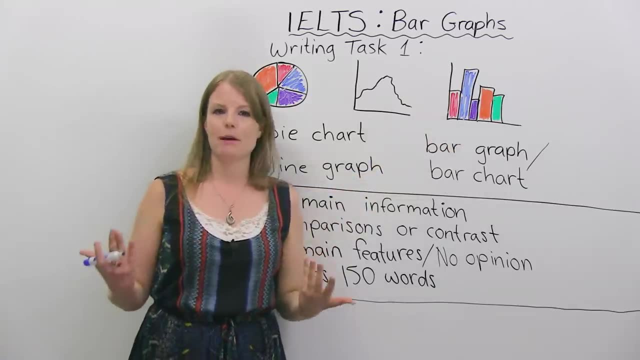 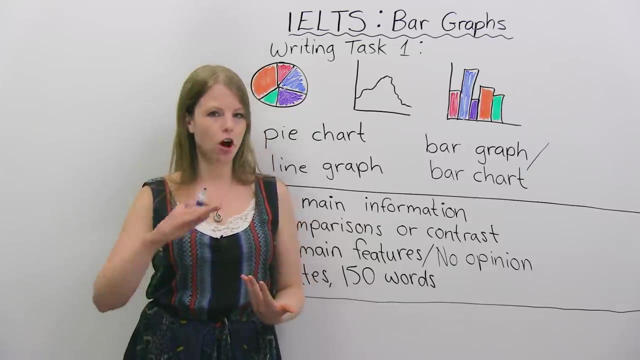 elementary school, secondary school, university, master's and like a doctorate or something. you do not write what you think about it. Okay, All you do is, in this type of question, you're just writing what you see and what it means. You're not writing your opinion. 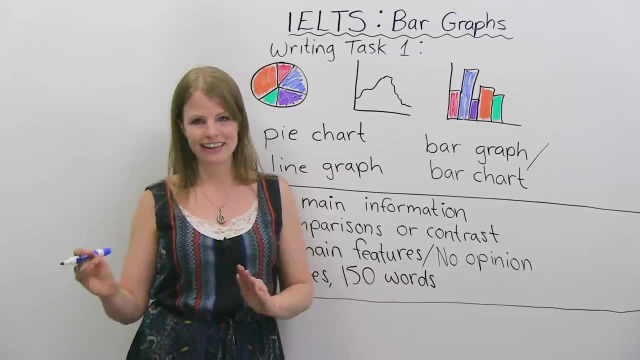 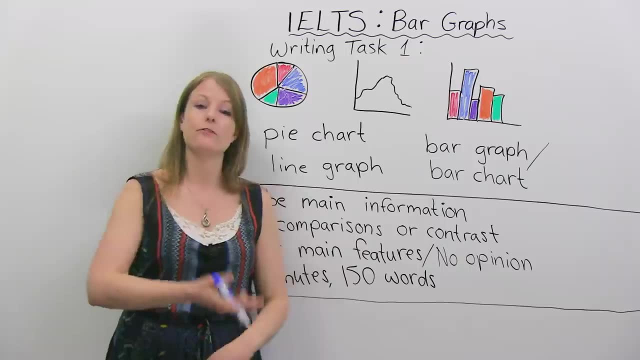 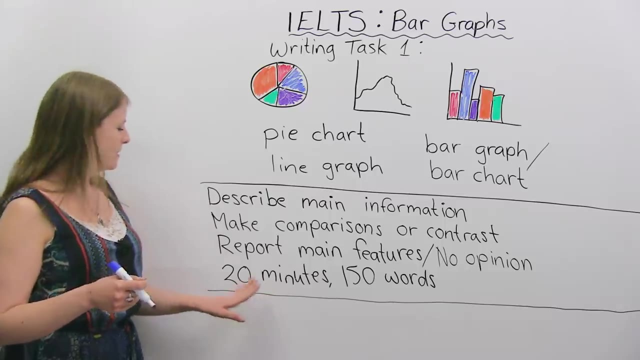 on anything, Okay, Because I think, or in my opinion, you'll actually lose marks for this. So in task one, no opinion, that's for task two. Okay. so for something like this, and we will look at an example question you have about. 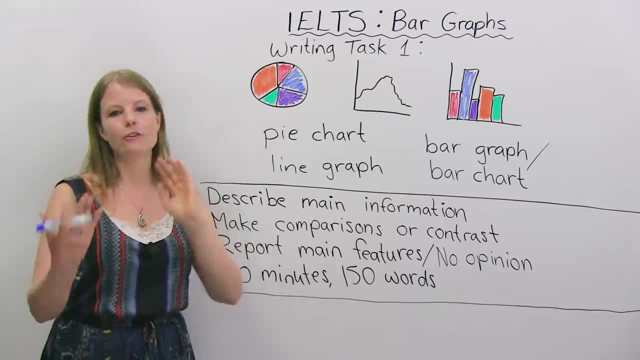 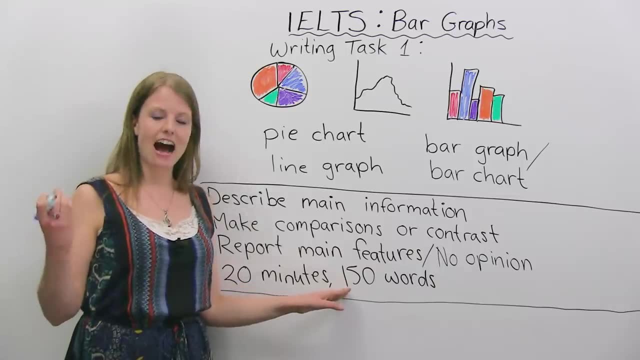 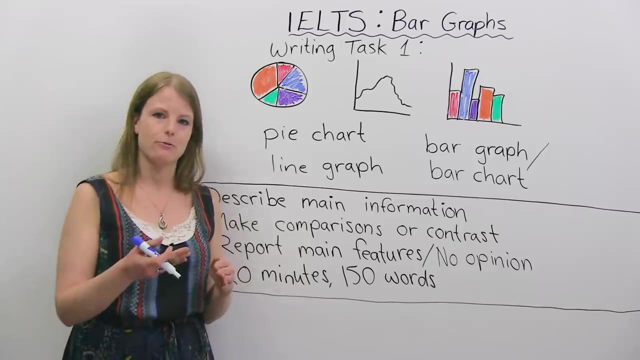 20 minutes. you know you're responsible for your timing, but something like this should take you about 20 minutes and you need to write at least 150 words. If you write less, you lose marks, So it's very important to write at least 150 words. There is such a 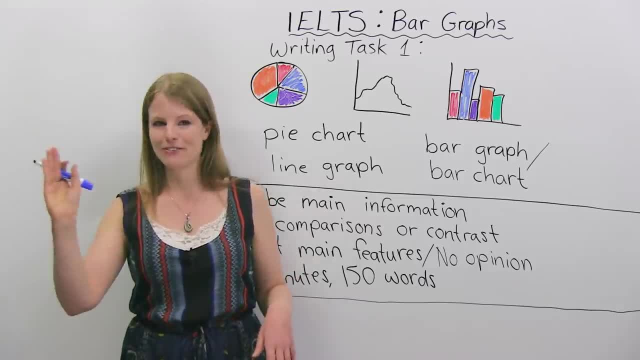 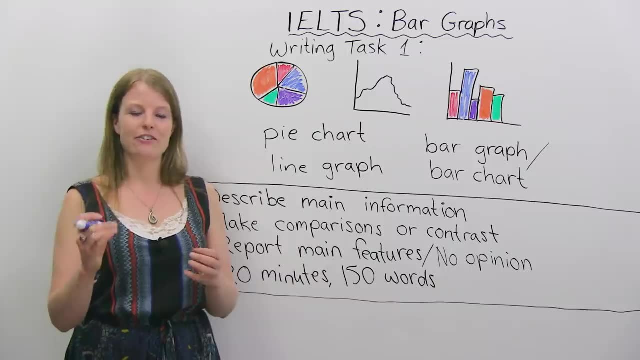 thing as too many words. so you don't have to write 800, that would be very bad. You know, writing 500 would be very bad. You're aiming for around 150 words. You know, maybe 170 is fine, but you don't want to write way too much either. 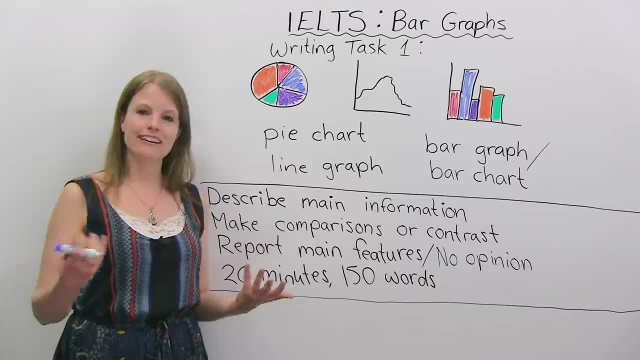 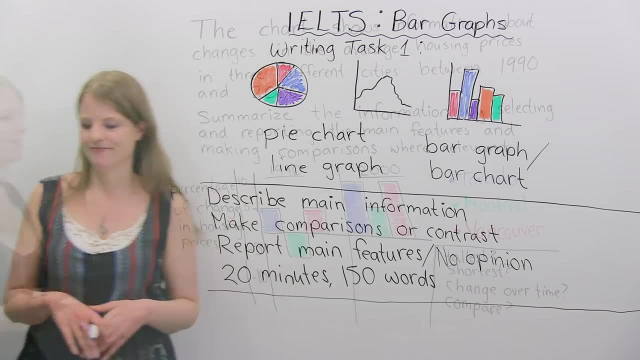 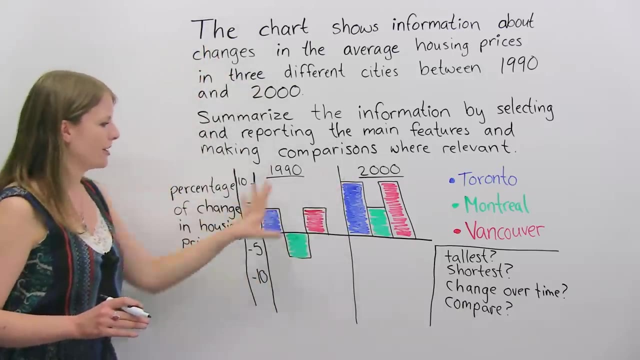 Okay so now we're going to look at an example of a question for this and some more tips on how to- How to write when you look at a bar graph. Okay so I have here an example of an IELTS question, So here's the chart and here is. 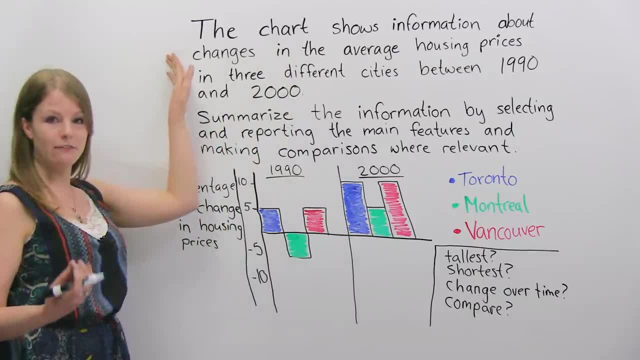 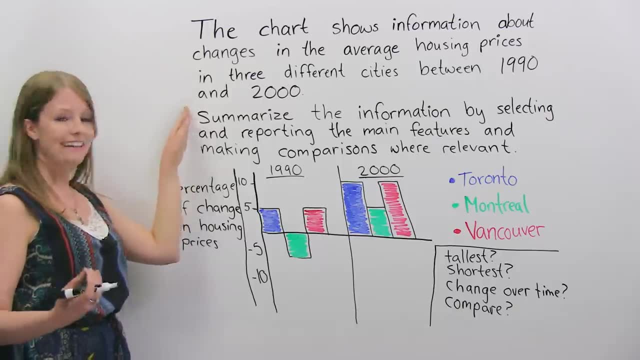 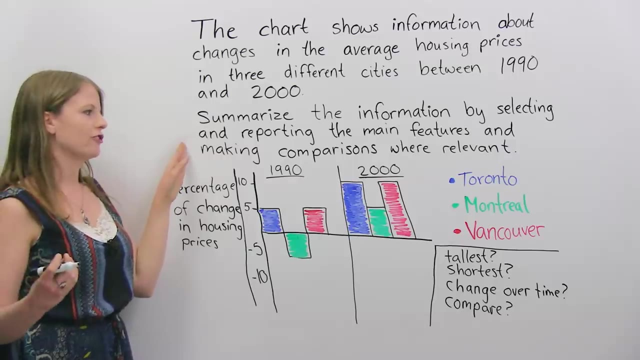 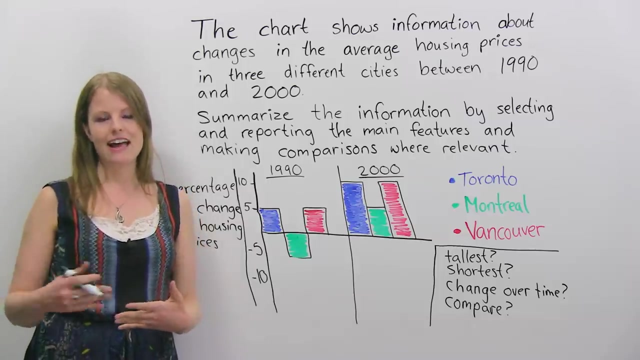 the question itself. It says: the chart shows information about changes in the average housing prices in three different cities between 1990 and 2000.. Summarize the information by selecting and reporting. Pretty instant answers. But why? Because it's pretty accurate. 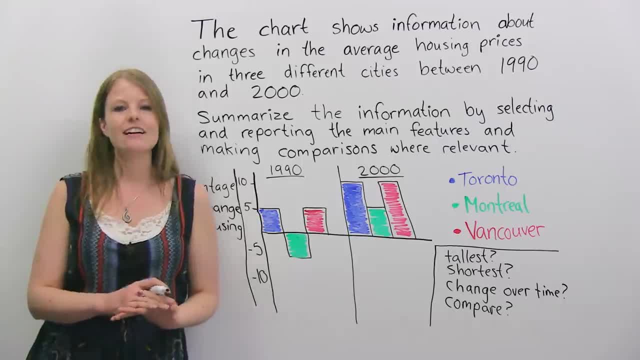 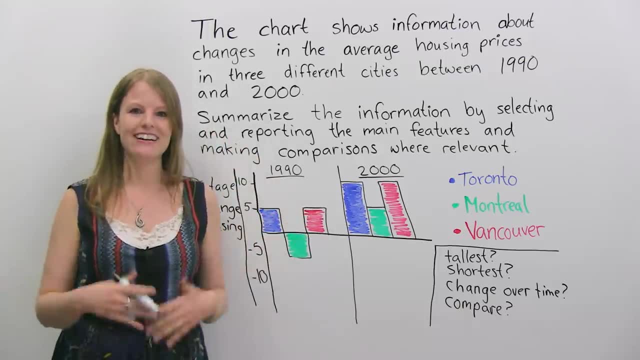 So for a question like this, you will. When I made a question, I wanted to write about 150 words, and that was important because I wanted to present a few facts. So the first thing you have to do is you have to write about 150 words And you'll show. 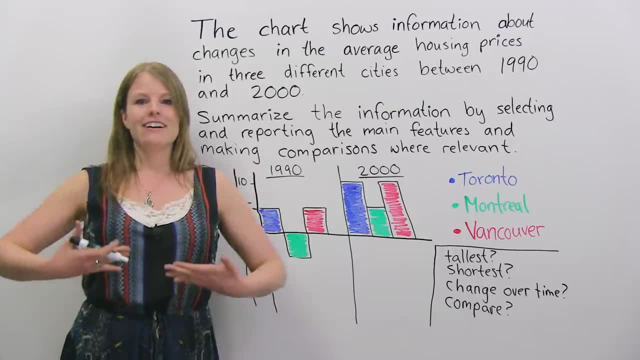 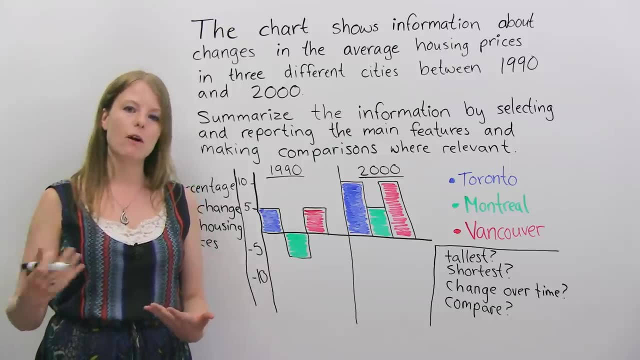 that you can't have thanks- erased answers, Right? So here's the question. It's simple And think about: what are you seeing? Don't just start writing. Think about what. can you actually see? What is happening here? Okay, 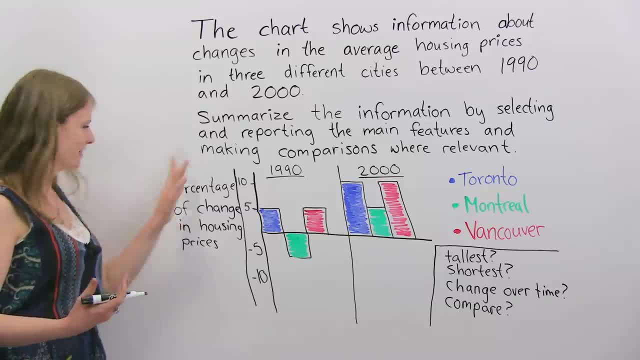 So, for example, here we have on this side this is called the Y axis- we have the percentage of change in housing prices. Okay, So I see the word here, percent, and I see the numbers 10,, 5,, negative, 5, and negative. 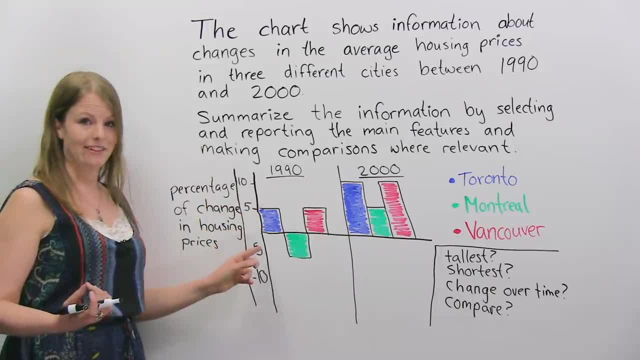 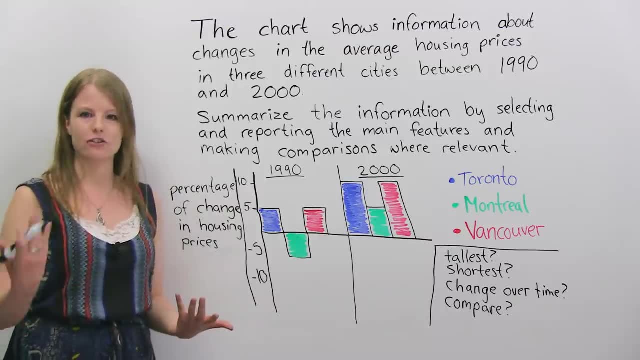 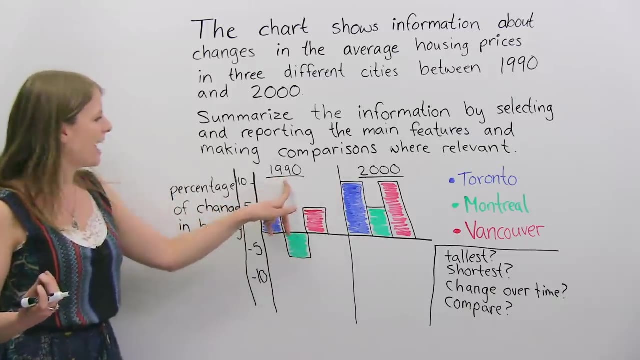 10.. So this is showing percent, Okay, And what kind of percent is it showing Housing prices, So the cost of buying a house? How has it changed over time? And then I can also look here and here. Okay, So we're looking at the year 1990 and we're comparing it to 2000.. 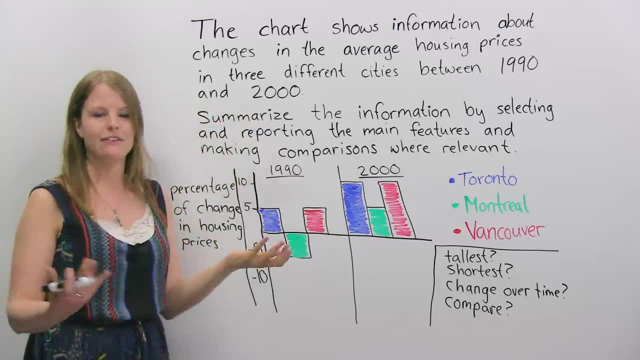 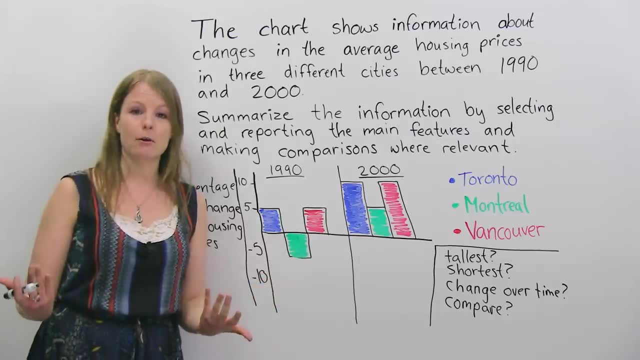 Usually the graph would also have a title. I didn't have enough space to write the title, but in terms of the visual you might see something like this. There are different types of bar graphs, So sometimes you'll just have you know, maybe one part of it. 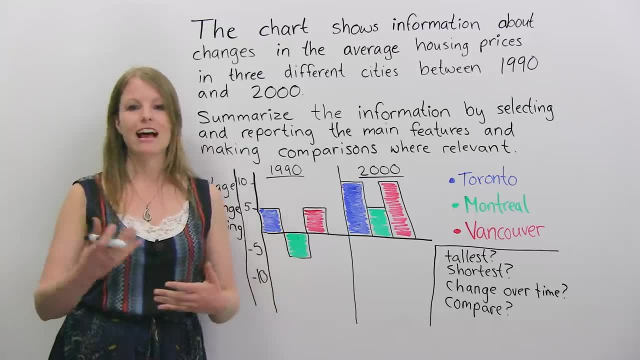 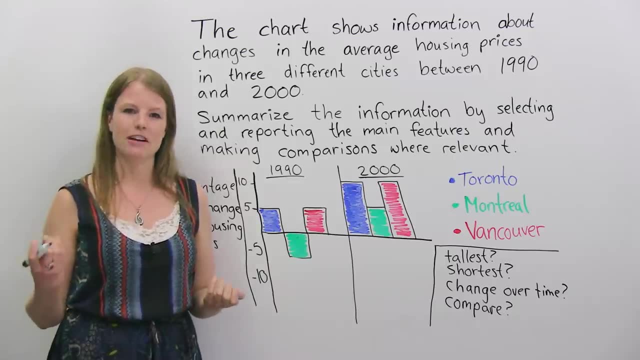 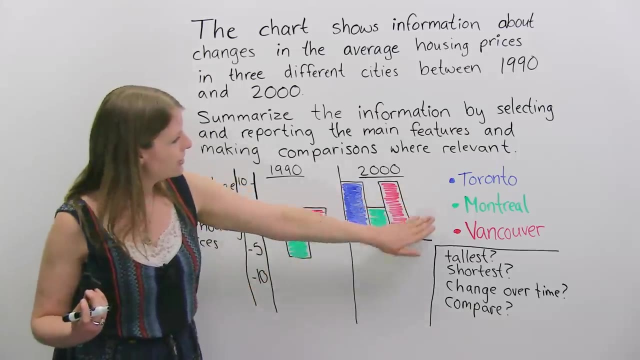 Sometimes you'll have multiple bar graphs you need to interpret. Sometimes you'll have a pie graph and a bar graph. So key here is: take your time to really think about what you're seeing. So in this case, we have three different colours- blue, green and red- and we have three different. 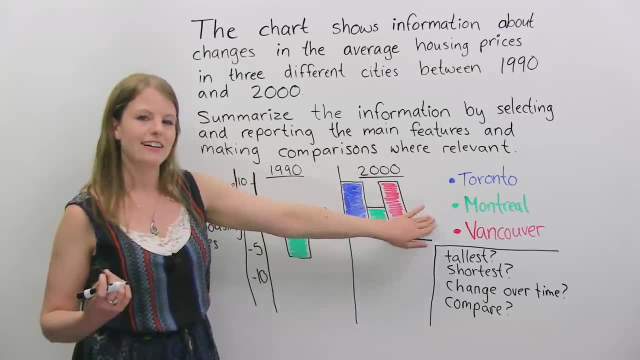 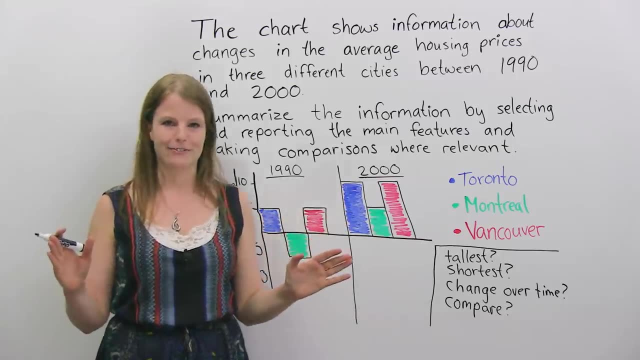 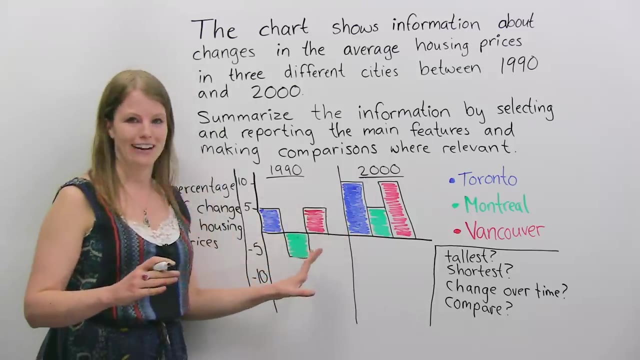 cities Toronto, Montreal and Vancouver, So I I made up this. by the way, This is not actually reflective of housing prices in these cities. I have no idea what housing prices are right now, so you know, don't take this as fact. 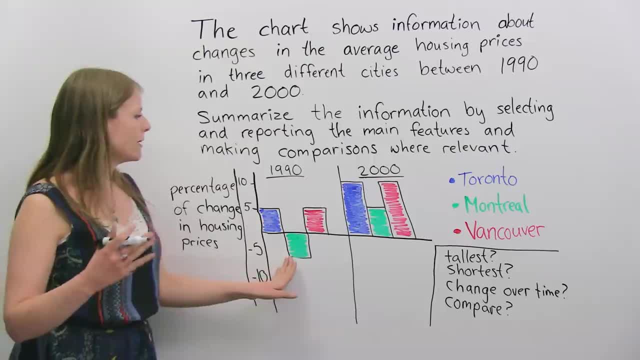 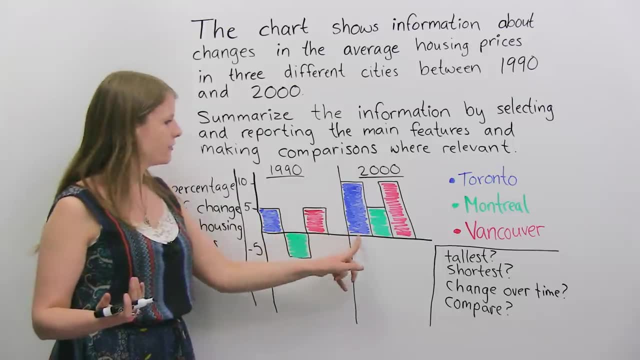 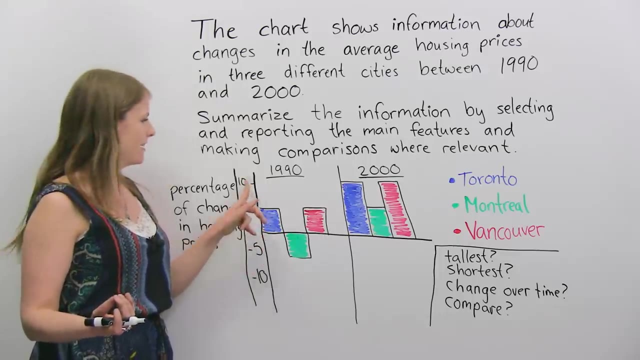 because it's made up numbers. So when you look at this, what can we see right away? Well, we can find Toronto. This is Toronto in 1990, and this is Toronto in 2000.. Okay, If I look here, this is about 5%. 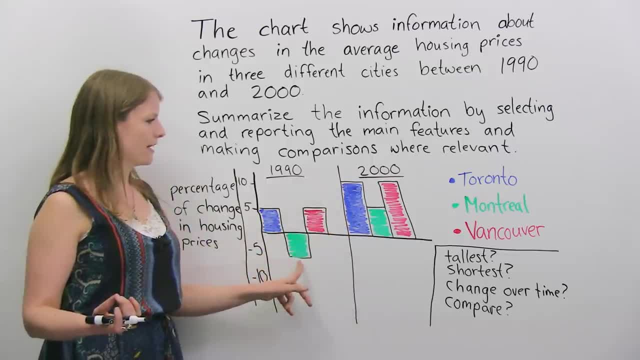 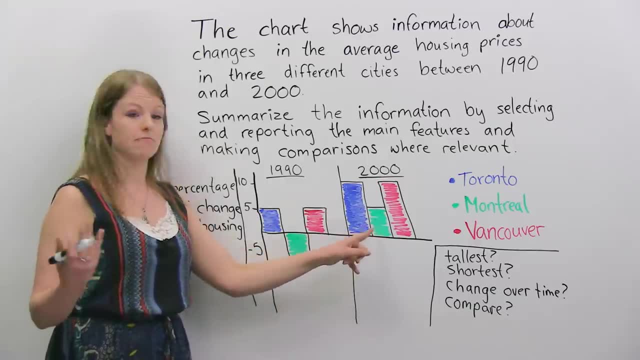 And here it's 10%. I can also look at Montreal. Montreal here is in the negatives. It's minus 5% compared to here in 2000,. which is 5%, so it's a positive number. And then we can look at red, which represents Vancouver. 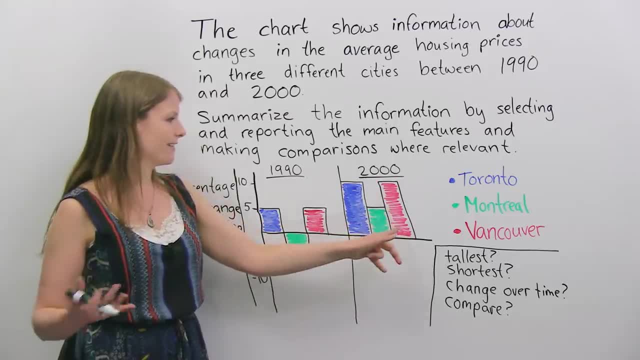 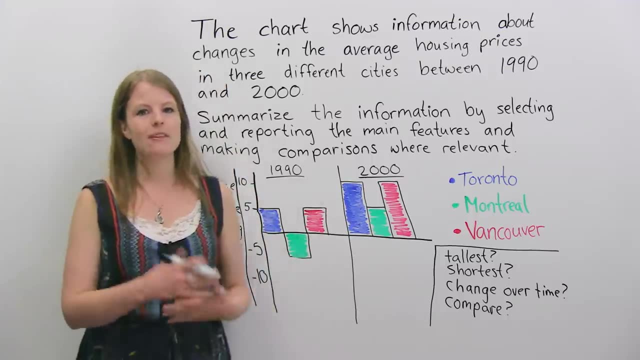 This is the same as Toronto. it's 5%, And this is again the same as Toronto: 5%. So you can start by asking yourself some questions: Okay, What are you looking at? You can look at the bars. 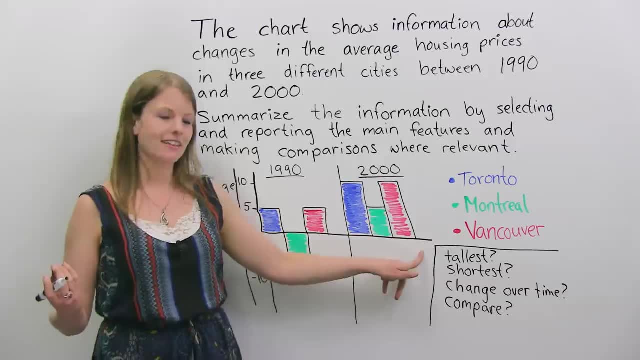 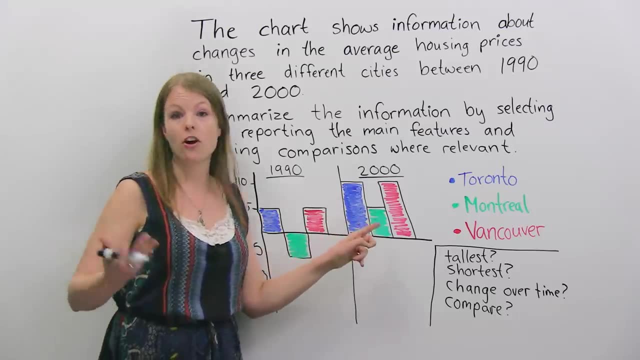 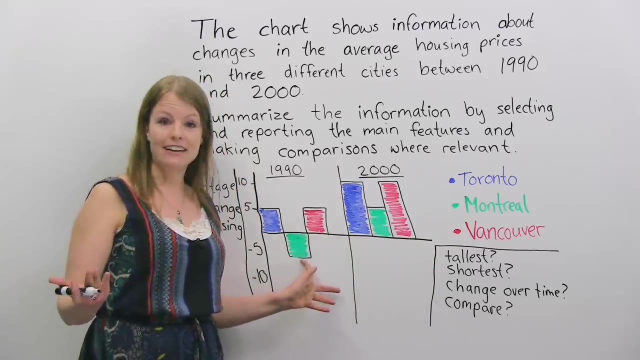 And think about which is the tallest bar. So in this case, the tallest bar in 1990 are both Toronto and Vancouver. In 2000, the tallest bars are also Toronto and Vancouver. We can look at the shortest bar. Well, in this case, in terms of negative, we see Montreal. 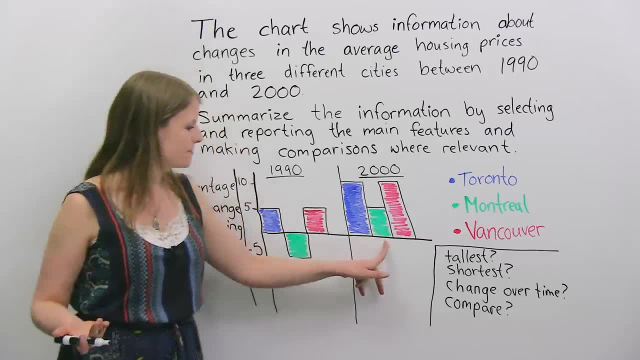 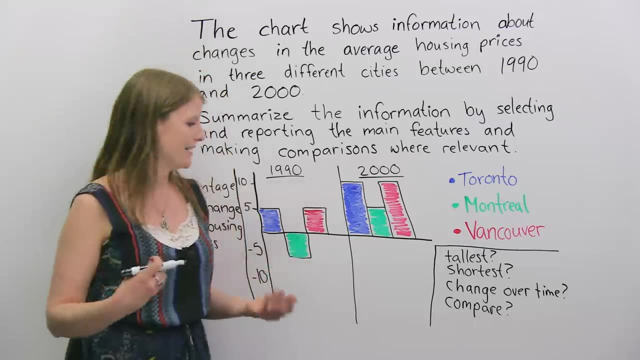 Okay, In this case, again, it's Montreal, So looking at which is the tallest and which is the shortest can are some questions you want to ask yourself right off the bat. You also want to look at change over time. Okay. 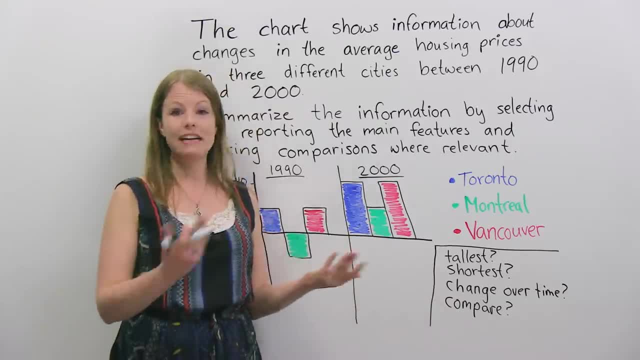 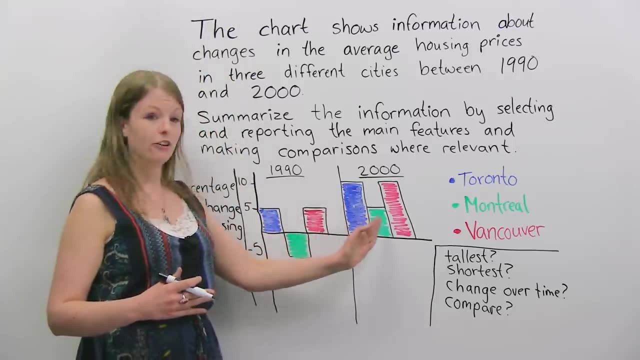 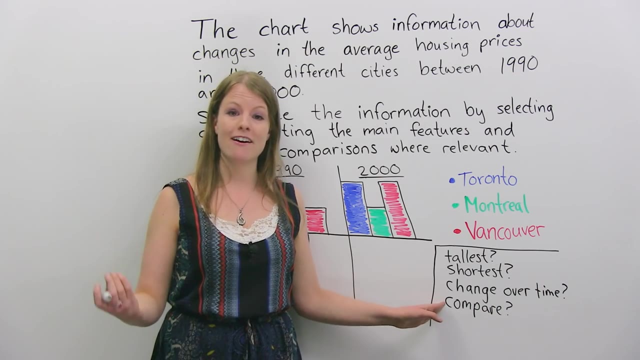 You know, how is this graph changing? Is something increasing? Is something decreasing? In this case, we see Toronto increased, Montreal increased and Vancouver increased. Everything has increased over time. You also want to compare. How are these bars the same and how are they different? 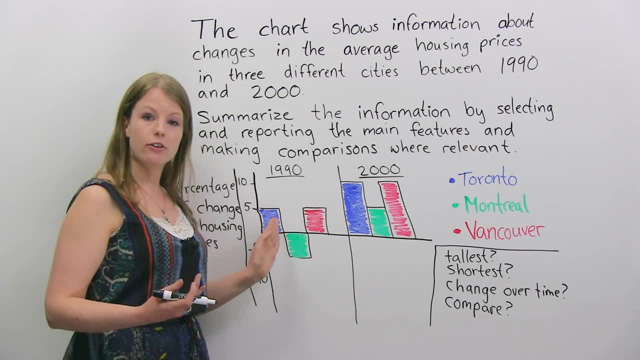 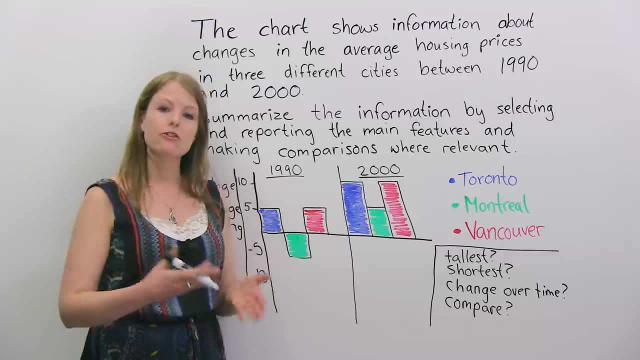 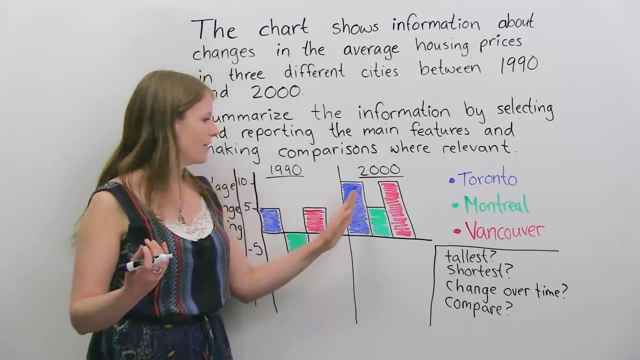 So I'll look Okay. In this case, Toronto and Vancouver are the same. Montreal is different. Toronto and Vancouver have both increased. Montreal has decreased. In this case, all three have increased, but Toronto and Vancouver are greater, you know. 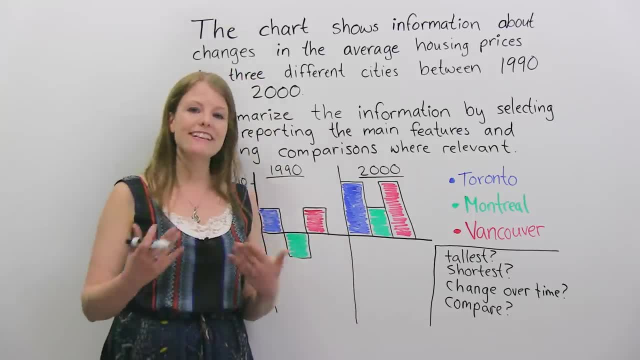 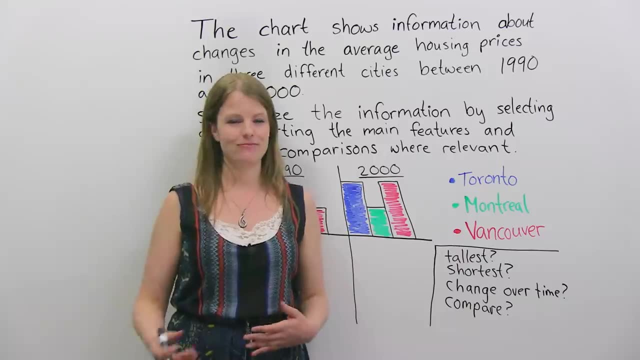 they show greater increase than Montreal. So noticing these types of patterns and just really analyzing what are you seeing will really help you in terms of your answer. So key point here: don't just write. take a minute to actually understand what you are looking at. 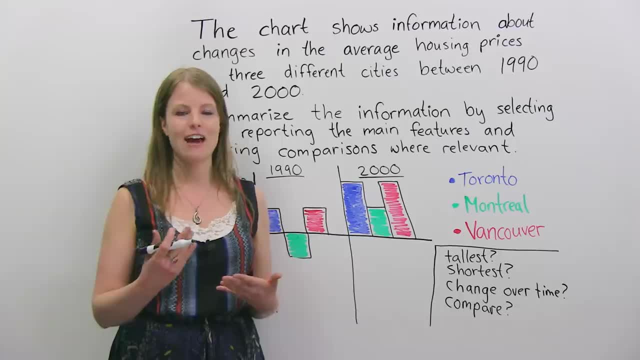 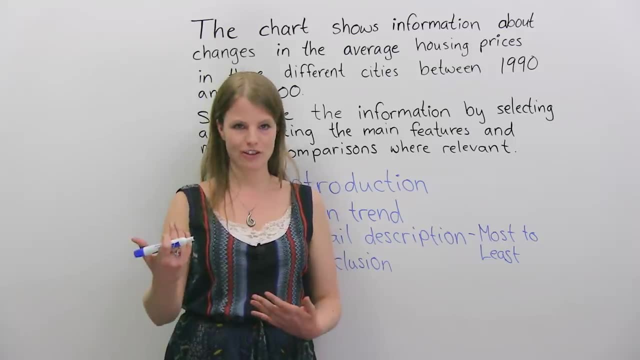 Okay, now let's look at some other tips on how to do, How to analyze a bar graph. Okay, so you've now understood what you're looking at. You've read the question carefully and you've also looked at the visual, in this case, a. 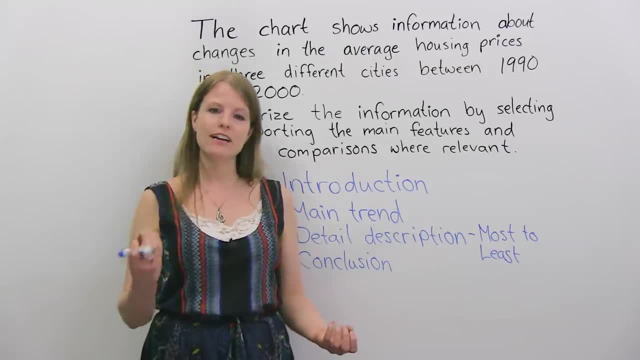 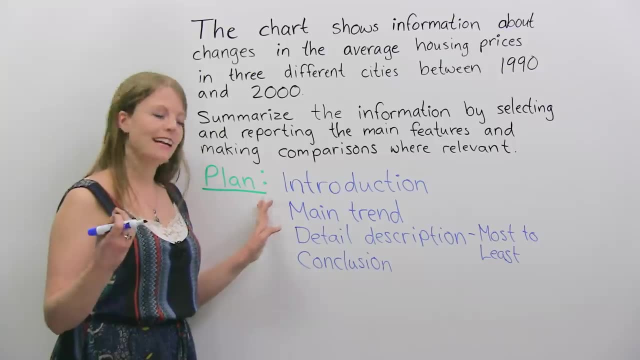 bar graph. So what do you do next? Well, it's a good idea to have a plan on how to do these questions. So, for example, What do you do next? What I would recommend is first write an introduction. Your introduction should not be long. 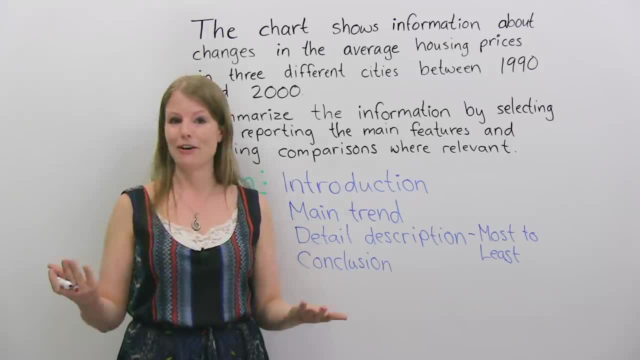 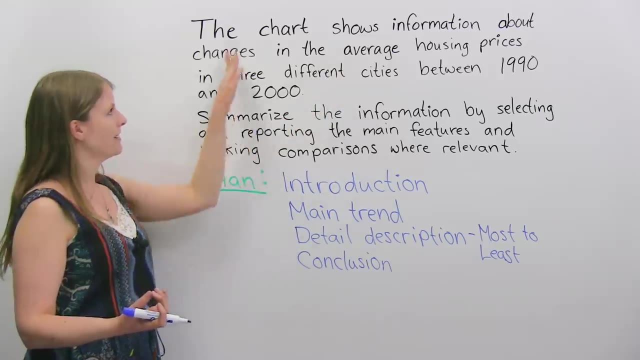 Okay, A lot of students they start the introduction and then they run out of time because they've spent too much time on the introduction. For this, you only really need to write maybe two sentences for your introduction. What your sentences should say in your introduction is it should pretty much say all of this. 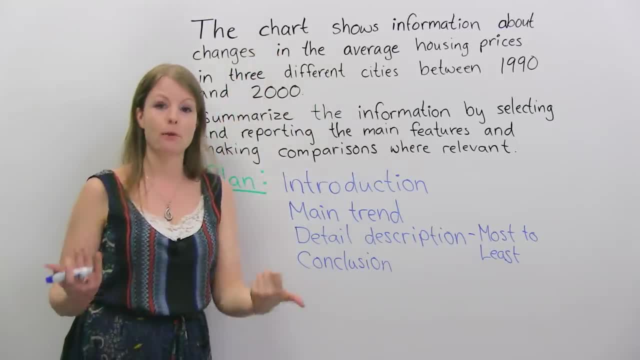 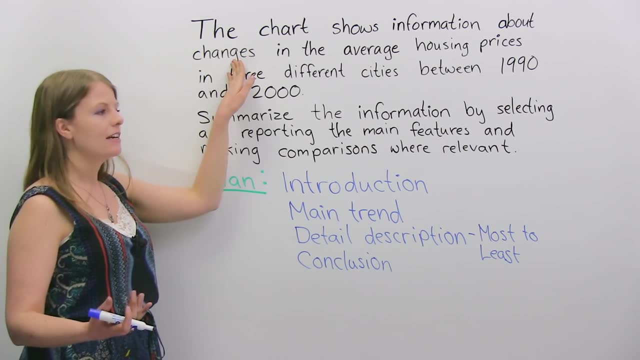 so you need to talk about what kind of chart it is. in this case it's a bar chart or a bar graph, And you can pretty much say all of this: information. Now, here's the tricky thing: You can't just copy what you see here. 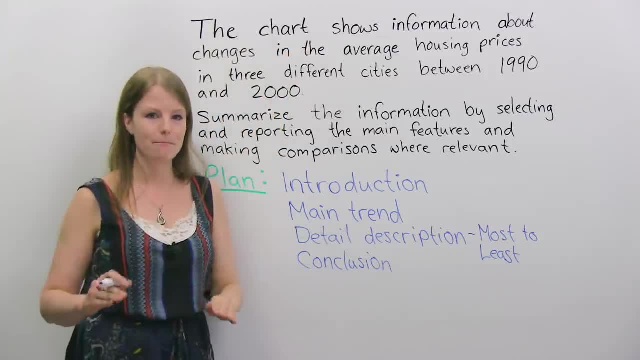 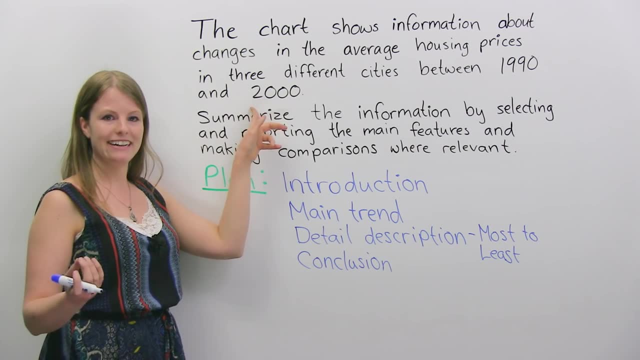 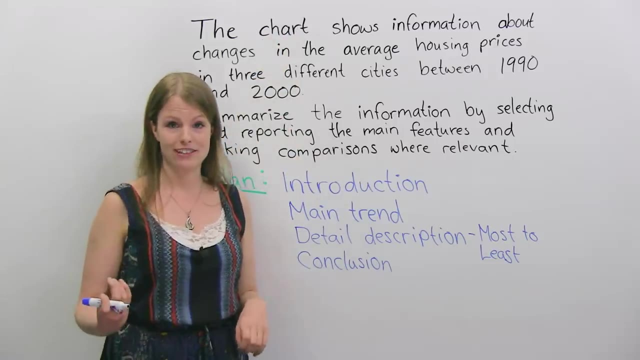 Okay, So in your answer your answer should not be. you know, the chart shows information about changes in the average housing prices in three different cities between 1990 and 2000.. If you copy the question you will lose marks. 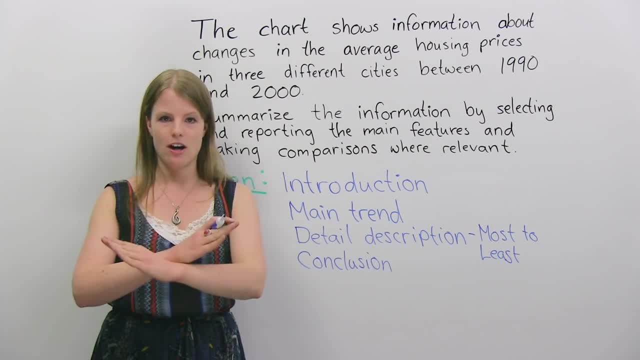 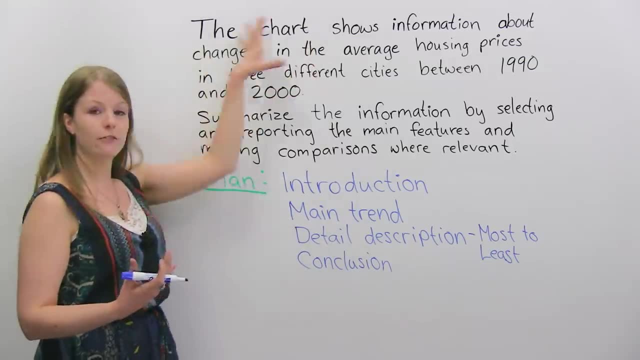 Okay, You will not show what you're capable of, so do not copy the words in the question. You need to use your own words to say all of this information. but use your own words, Okay. So one way to do this, instead of saying: 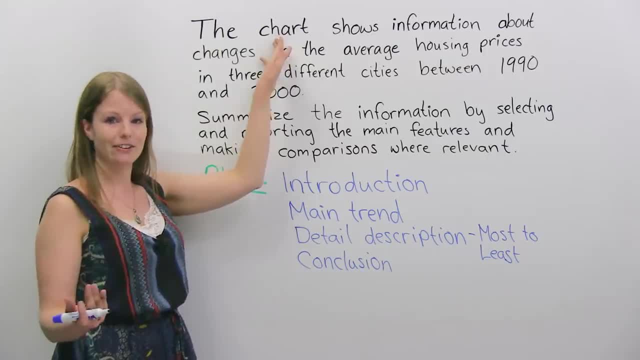 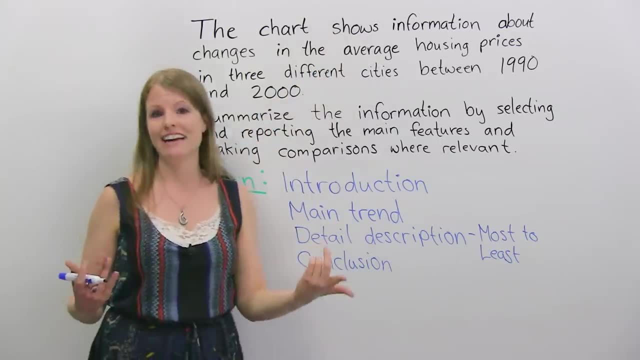 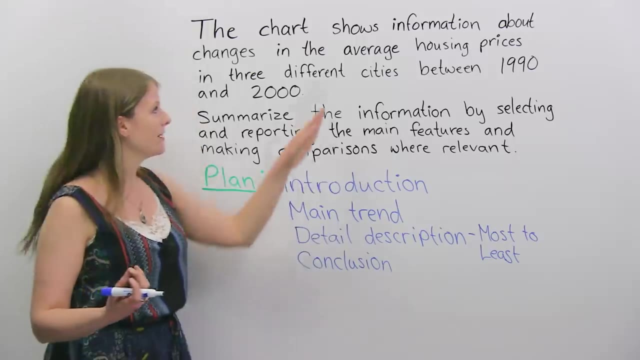 If they say chart here, you can change that to bar graph. Okay, Instead of using the word show, maybe you can use the word demonstrate or indicate, or, you know, represents, Illustrates. So there's a lot of great words you can use instead of the word show. 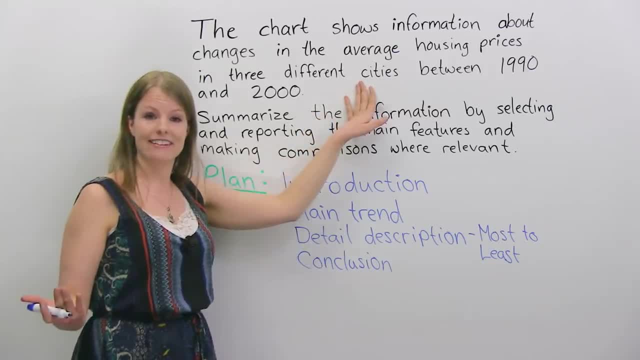 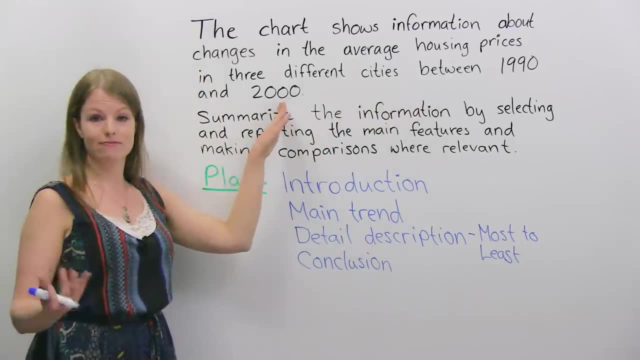 In terms of the three different cities. you can actually name the cities. In this case, we looked at Toronto, Montreal, Vancouver. You know you'll also have to include details about the dates, but you can change some of these words around. 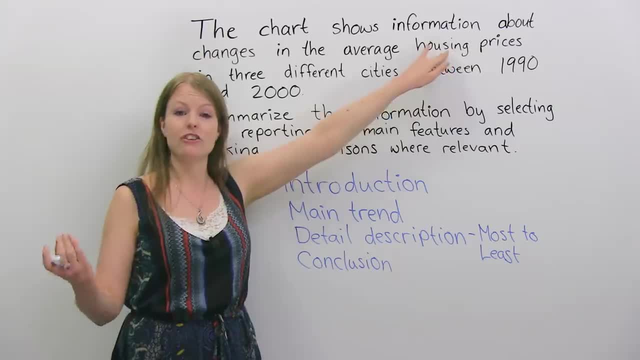 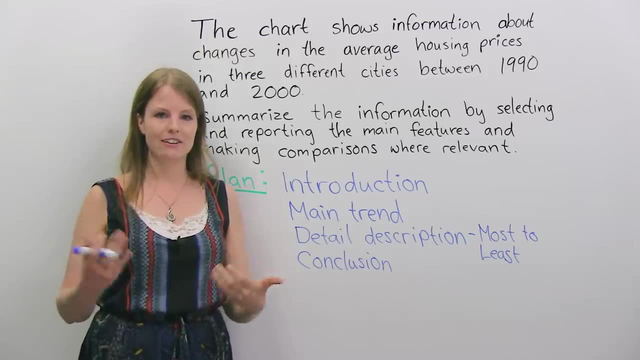 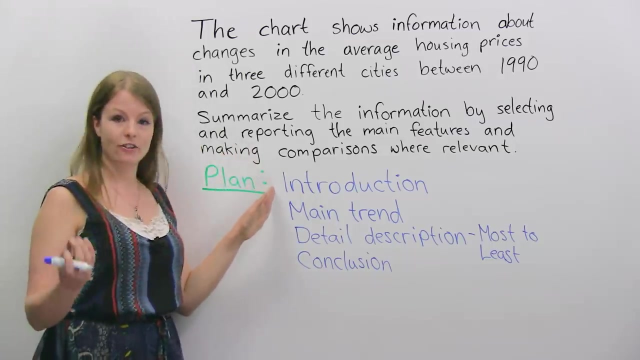 Instead of average housing prices. maybe you could change that to the price of housing, You know. So there's different things you can do. Main point here is change the wording and change the sentence structure if you can. So that's key in your introduction. 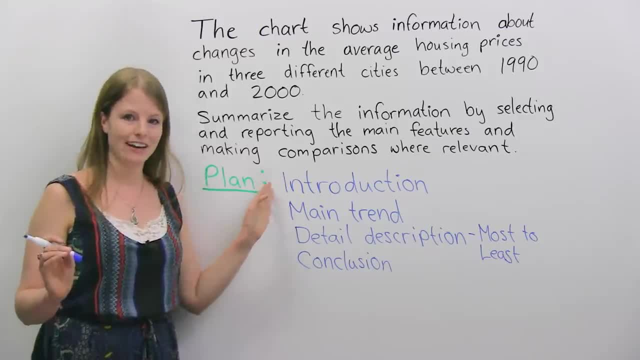 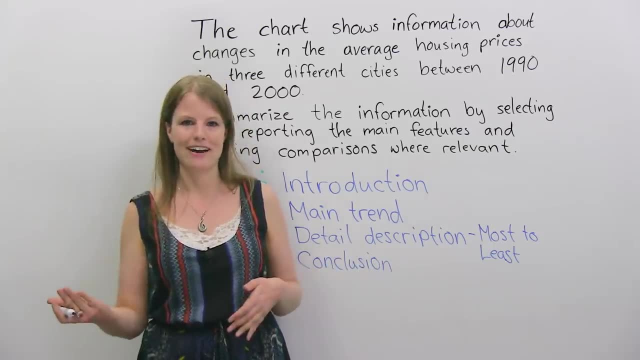 Again, you are not giving your opinion here, Okay. So whether you think, oh, it's great that you know all these Canadian cities, you know their housing prices are going down, you don't give your opinion about it. 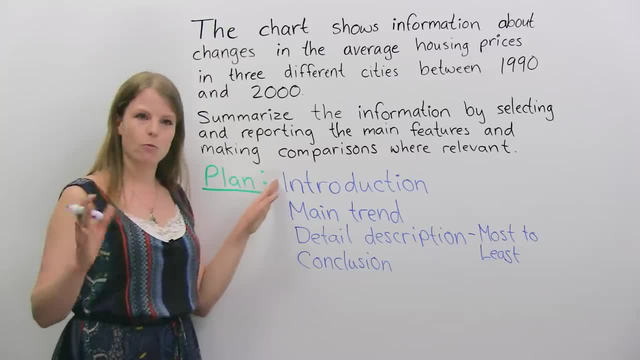 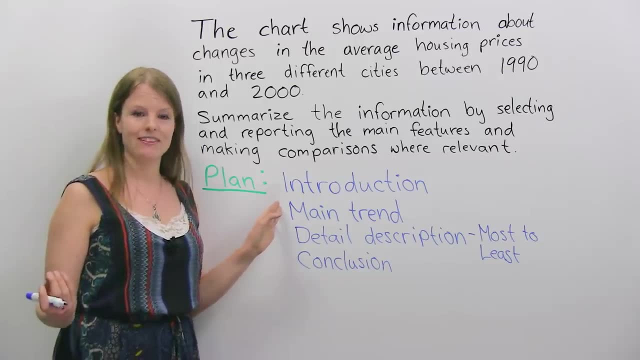 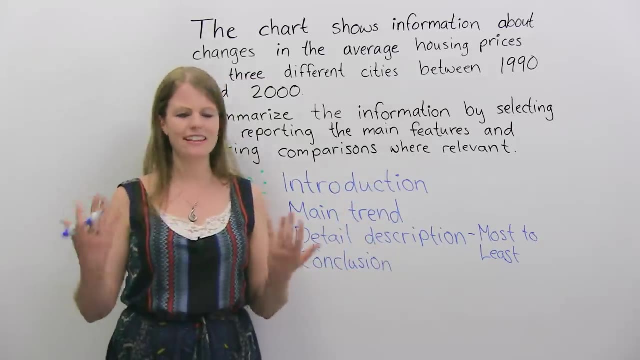 Okay, the next thing you should do. So your introduction is Again About maybe two sentences. You can now give a sentence or two about the main trend, you see. So the main trend is the most important, or the most you know. 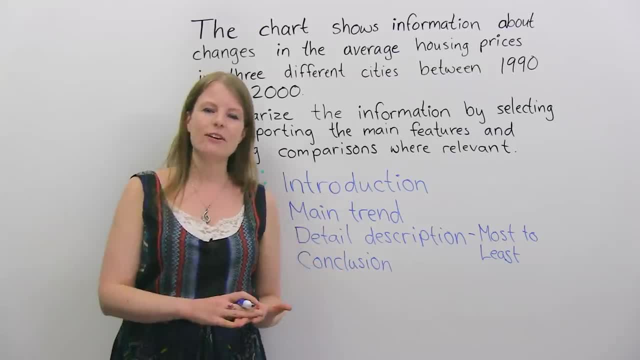 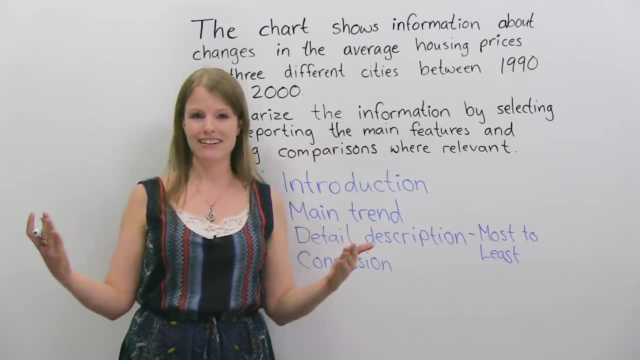 The thing you see that is kind of like the biggest thing. So in this case we looked at housing prices of Vancouver, Toronto and Montreal. One thing that was a very big trend is that everything increased. All of the cities increased over time in terms of their housing prices. 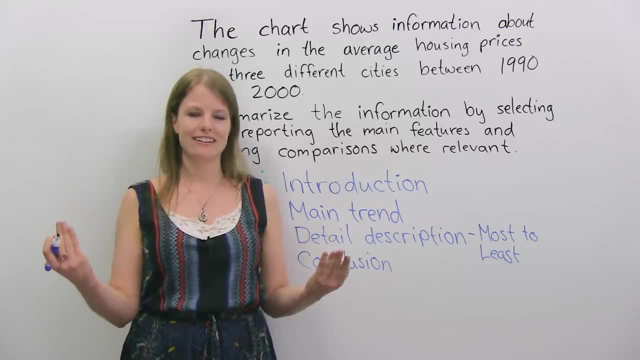 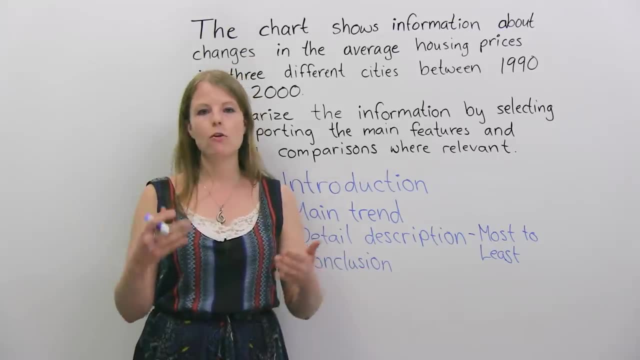 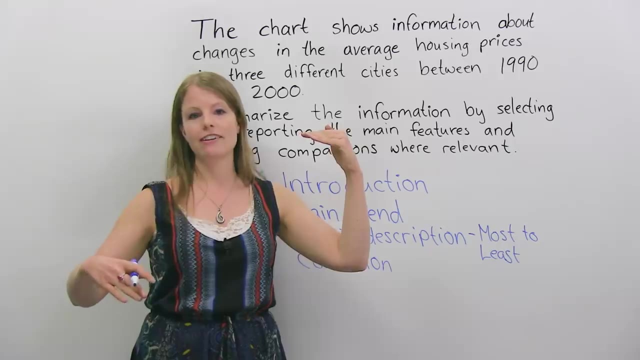 That's a main trend. So anything that's a big pattern that when you look at you notice: okay, all of these things show the same pattern, or maybe you know it might be that one of the main trends is that Vancouver is the most expensive and Montreal is the least expensive. 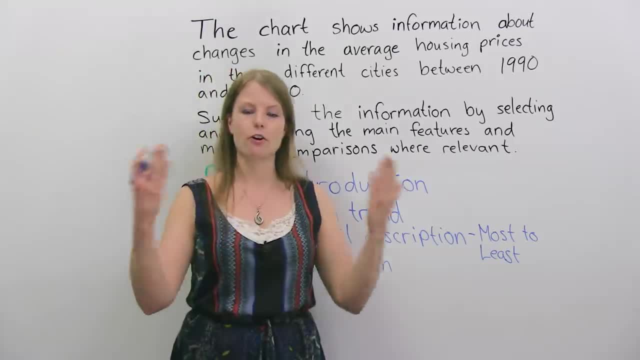 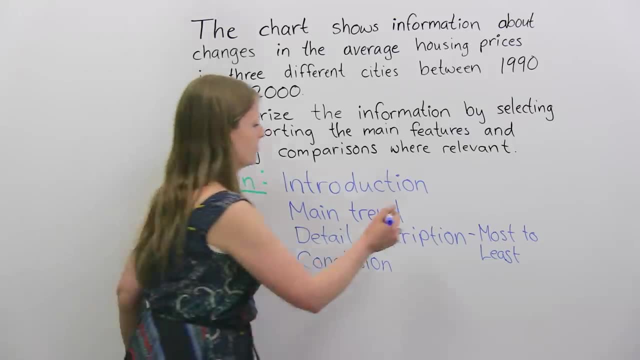 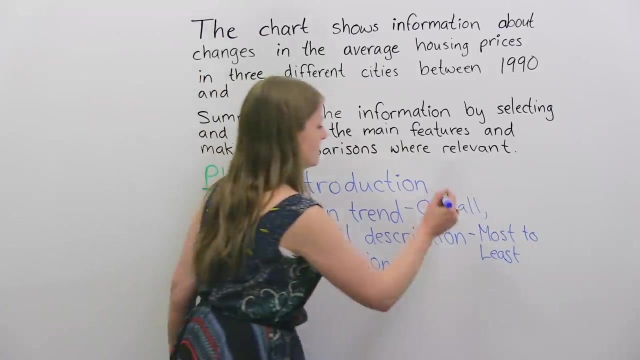 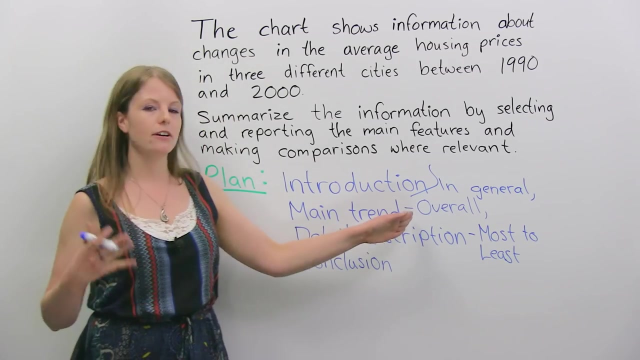 These types of things are things that you can write about overall. So, in terms of when you're talking about main trends, there's two great words to use: Overall, or- and I'll just put that here- in general. So these are two great words that can start off this sentence, where you show off what 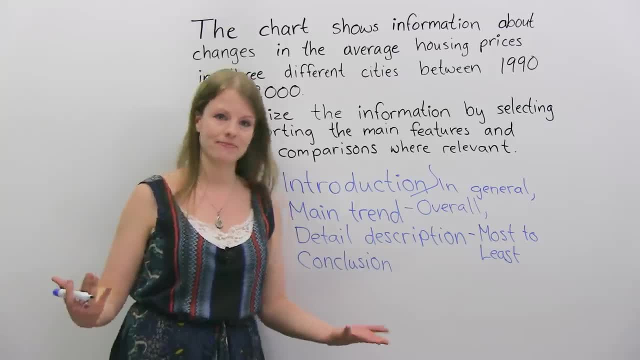 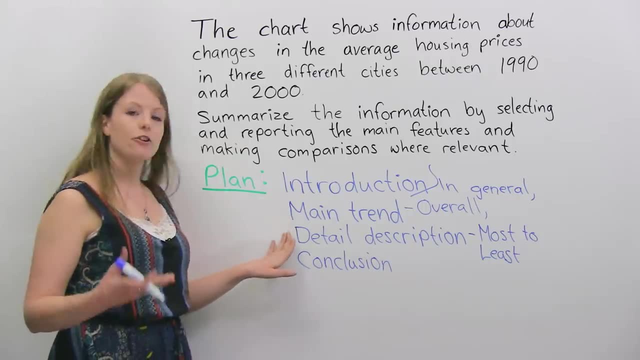 is the big picture or the main idea. Okay so, And that should be, maybe, you know, two sentences After you finish the main trend, then you're going to have a new paragraph And in this new paragraph is where you're going to say most of the details. 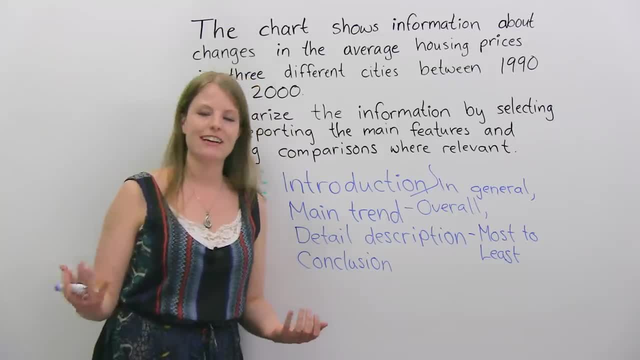 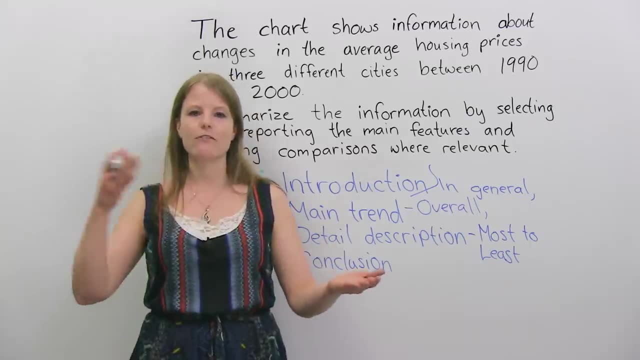 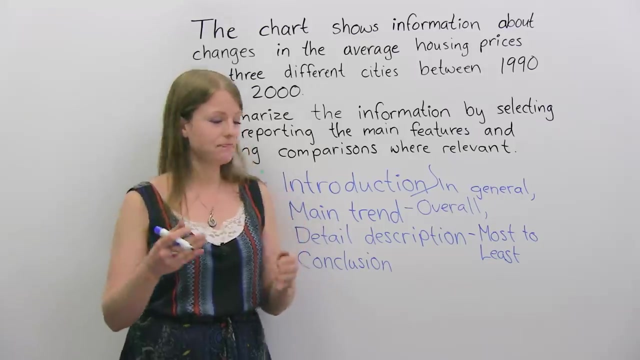 Okay, So you're going to say specific numbers, You're going to, you know, really do comparing and contrasting between them: Toronto is like this, Vancouver is like this, Montreal is like this- And you're going to look at each thing individually and you know, together. 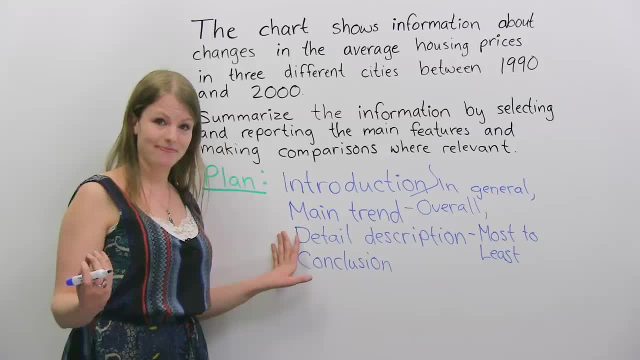 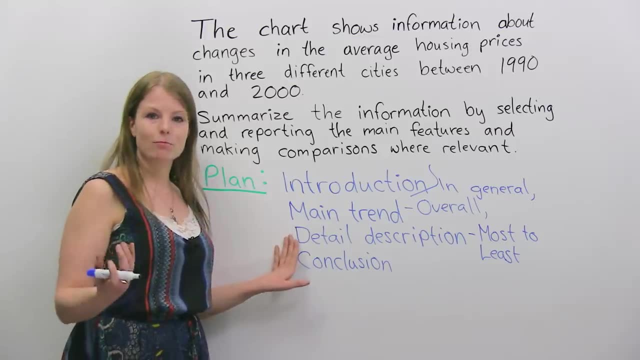 So in this case, the key here is detail. Okay, So you want to have as much specifics and details, As much detail as possible, And you're pretty much summarizing what you see, but paying attention to specific numbers and specific details. 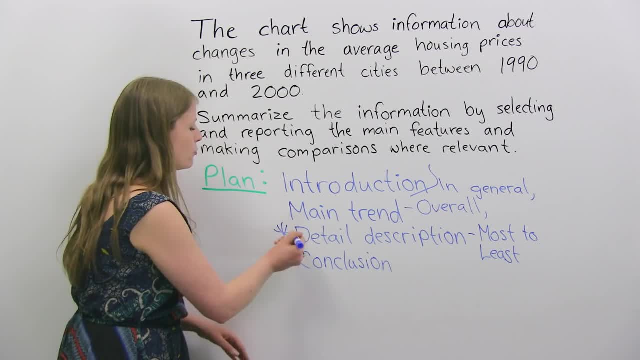 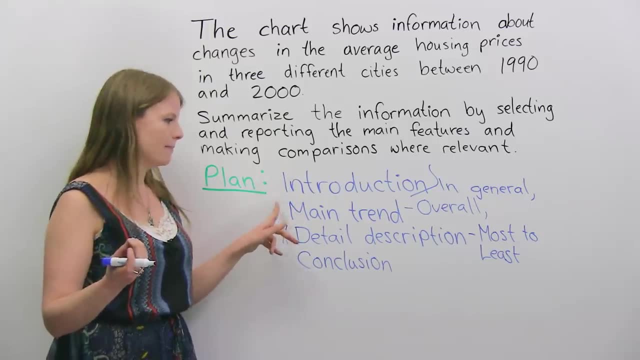 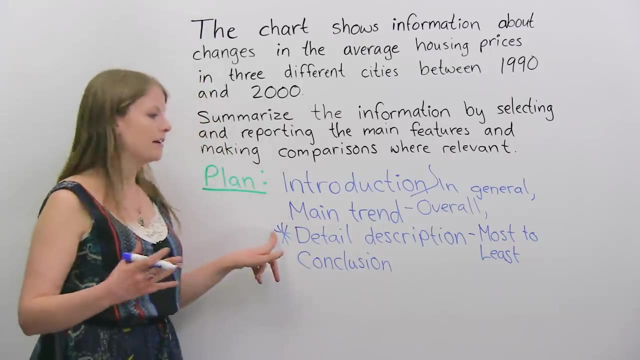 A good tip with this. So this is where the majority, your biggest paragraph, is going to be. here. You can introduce, You can use your introduction and the main trend as one paragraph, if you want, or two, but your biggest paragraph is going to be the detailed description. 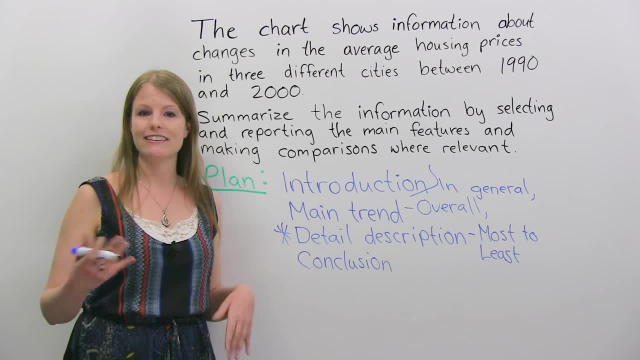 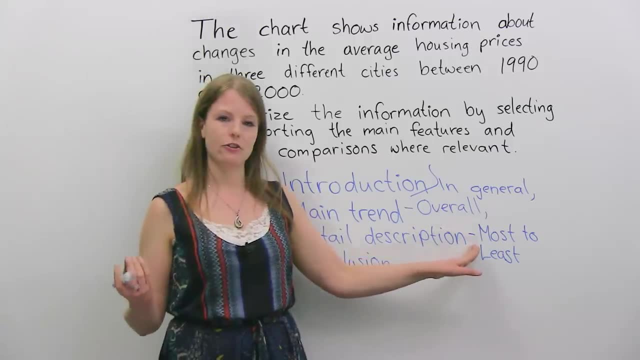 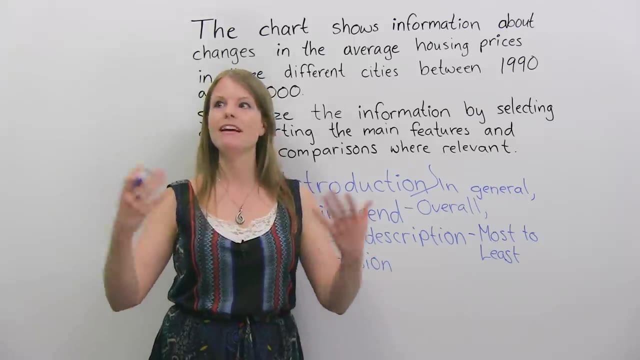 Okay, This should be, you know, maybe five, six sentences, so it should be a lot longer, maybe even more. In this case, what you want to do is you want to write the most important and talk about it, or the biggest trend you see, and then go smaller to something that maybe isn't so. 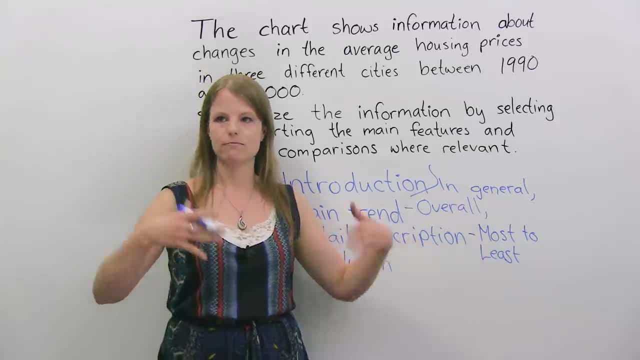 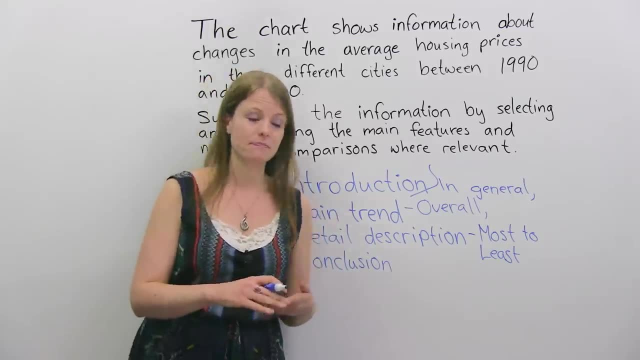 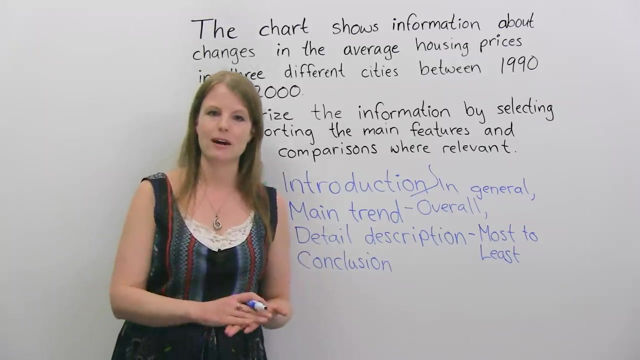 important. So you're paying attention to the most important information and then you're going to the least important information- Okay, Including it all- And finally you can write a conclusion. It's not necessary, but it does wrap up your answer quite nicely and your conclusion can. 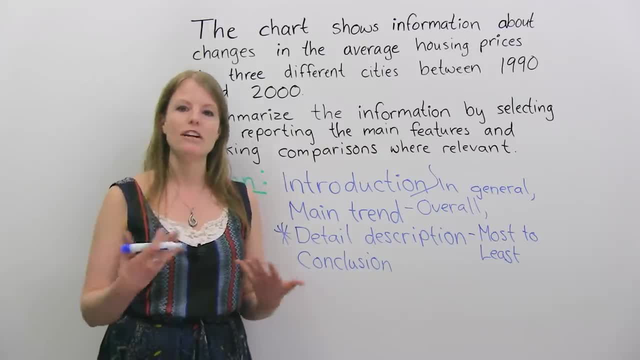 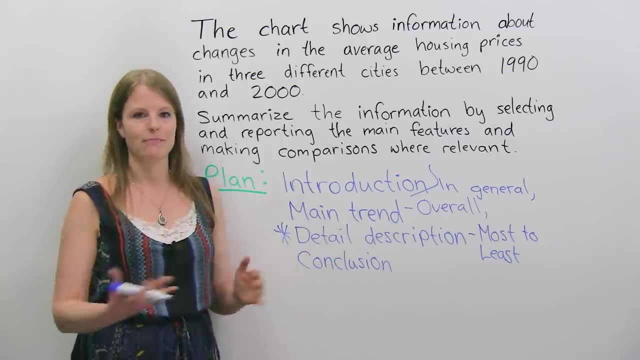 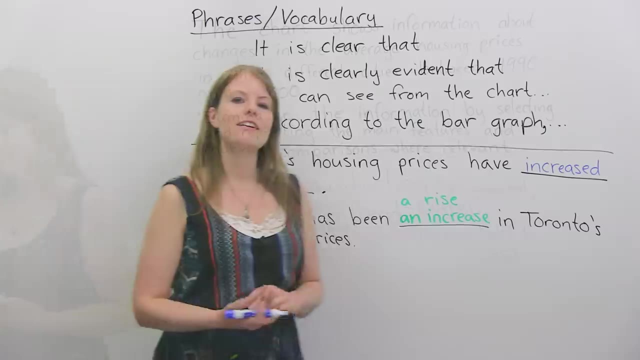 just be one sentence, just explaining. you know what you saw in one sentence. So this is a good plan on how to write- How to write when you're describing a bar graph. All right, so now let's look at some more tips on how to do this type of answer. 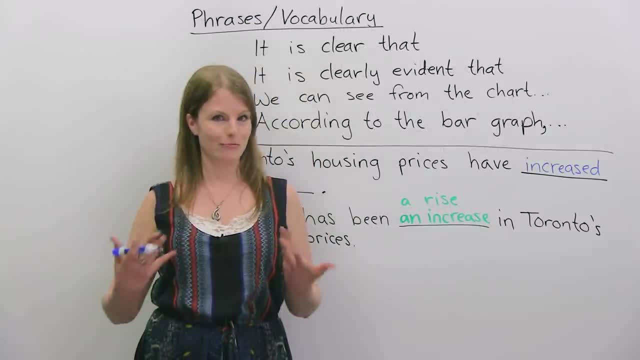 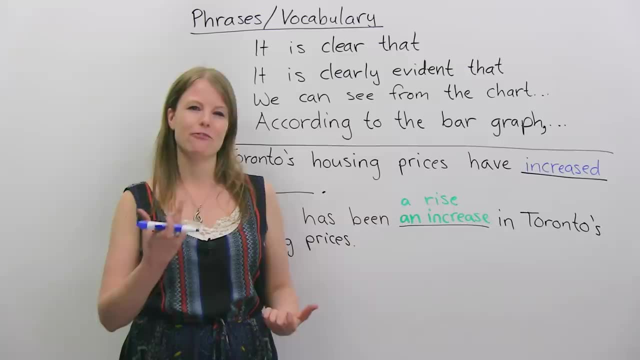 Okay, One way to deal with you know you're going to be very nervous, probably, or maybe a bit anxious while you're writing the IELTS. one way to deal with this, with the writing, is to actually have some phrases memorized that you're used to using. 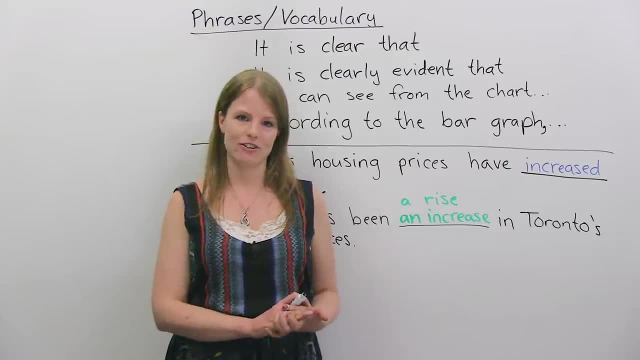 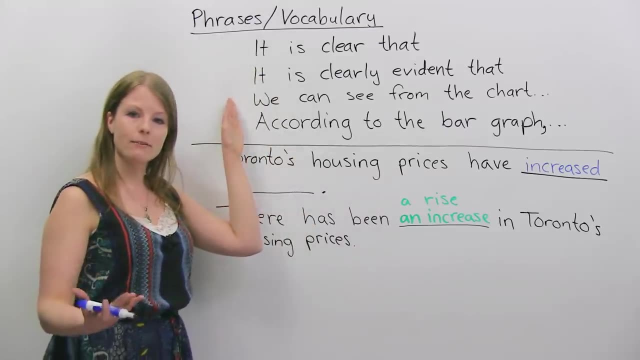 This can help you save time and, as well, this can help you with the word count on the IELTS, because you need at least 150 words. So I have here some key phrases. You don't have to memorize all of them, but maybe pick one or two and you can use this. 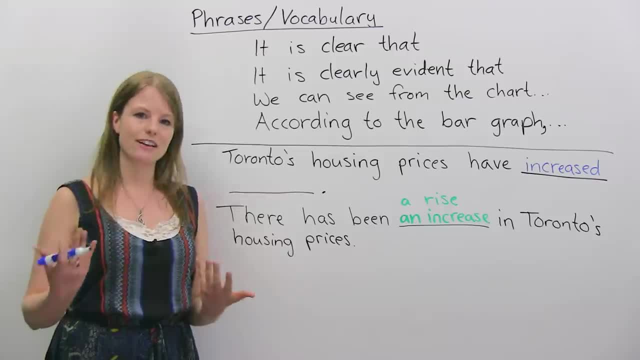 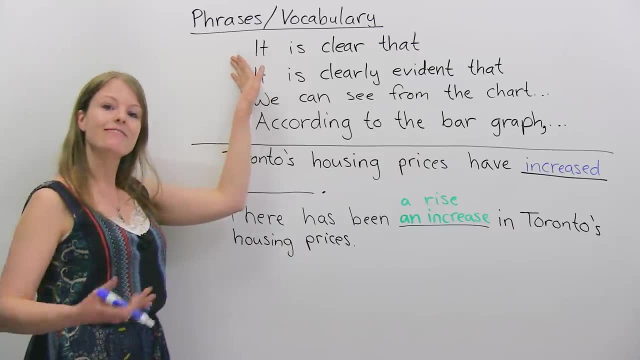 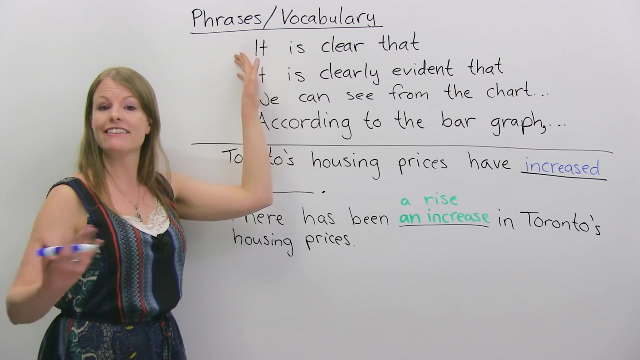 on the IELTS. You can practice these and you know they can really help with your describing of a bar chart or a bar graph. So, for example, it is clear that If we looked at the example we were just using, it is clear that Vancouver has had the greatest 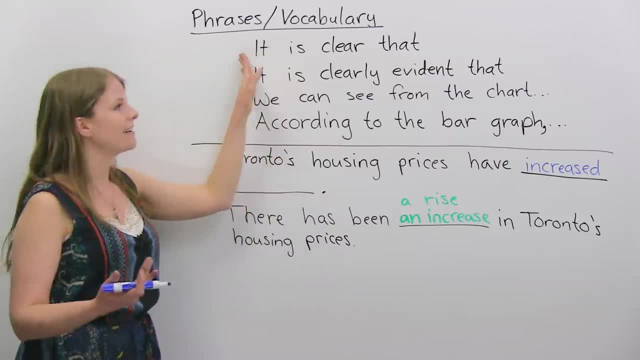 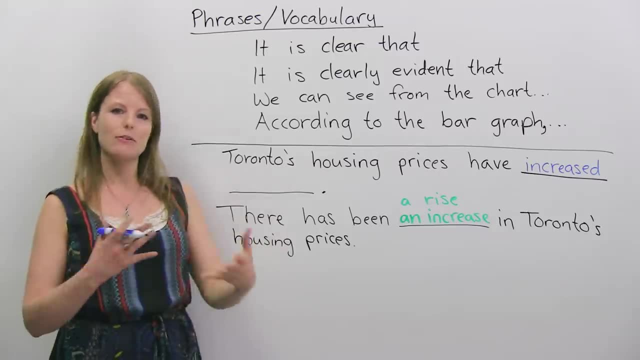 increase in average housing prices. It is clear that Montreal has, you know, increased a little bit. Okay, So pretty much, you can use this as the beginning of your sentence. You can use this as the beginning of your sentence to talk about some of the patterns. 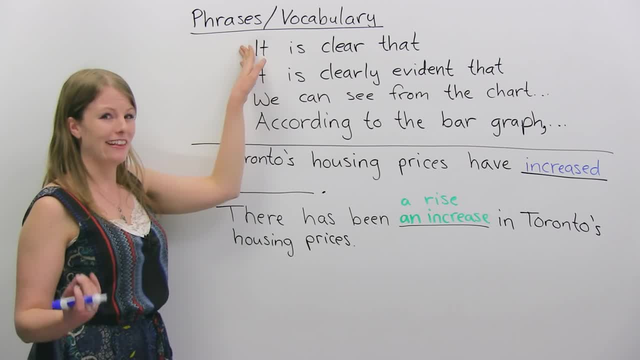 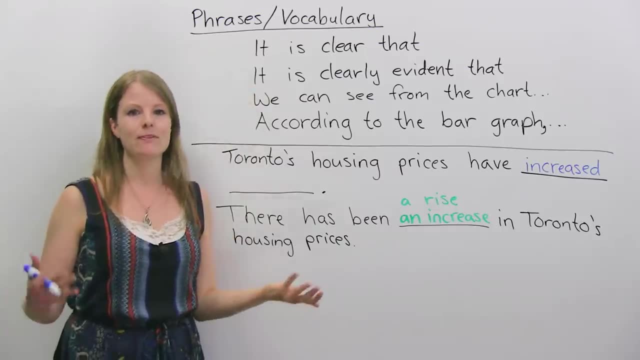 you're seeing. What's even better than this is the next one. It is clearly evident that. Why is this better to use? Well, for the simple reason of it's longer, and you need to, you know, have 150 words. 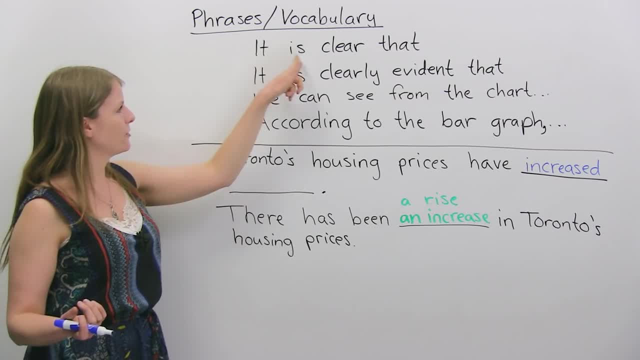 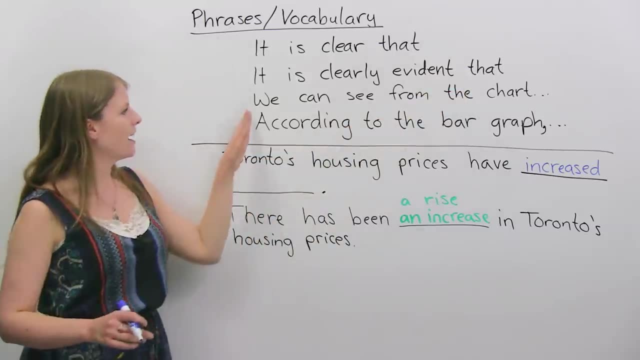 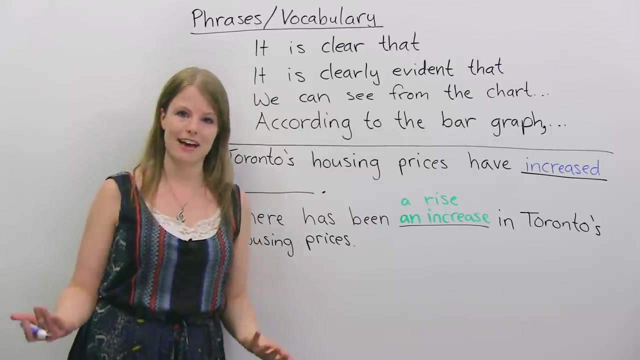 right. So each word you use counts. So let's count One, two, three, four versus one, two, three, four, five. So you're getting an extra word in there. Use the next one. We can see from the chart that. or we can see from the bar graph that again you just. 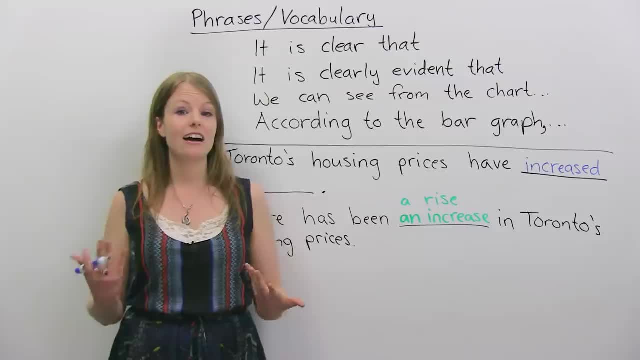 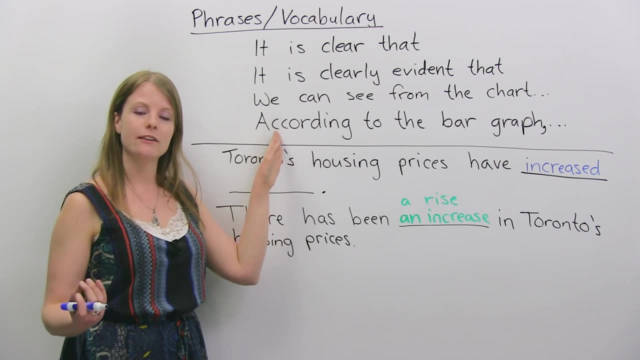 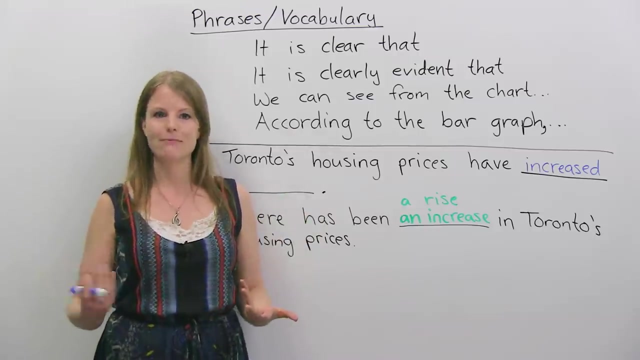 insert the information, whatever it is that you're looking at. you know this is a way to introduce what you're seeing. You can also say: according to the bar chart or according to the bar graph. So these are great expressions you can use which will really help you save time thinking. 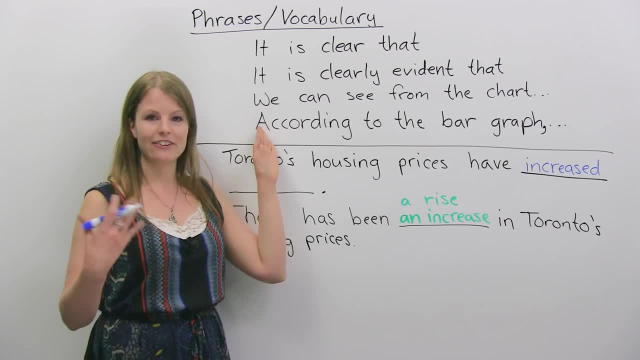 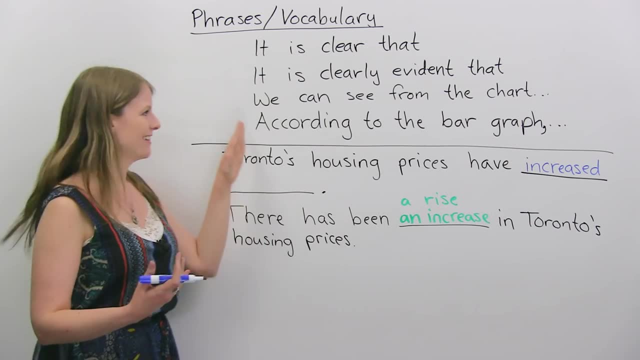 about how to start a sentence, But you know, here's a. Okay, Just a bit of caution: Don't reuse the same one again and again and again. You don't want to use this for each sentence you're writing. 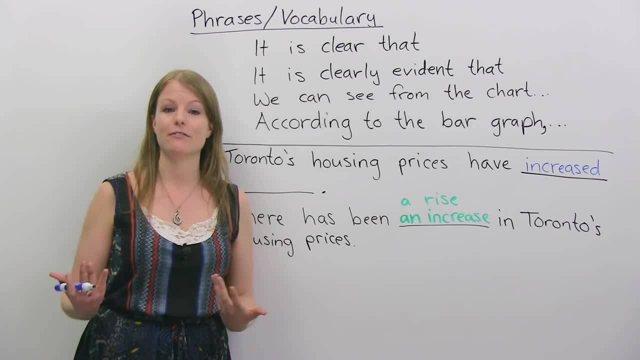 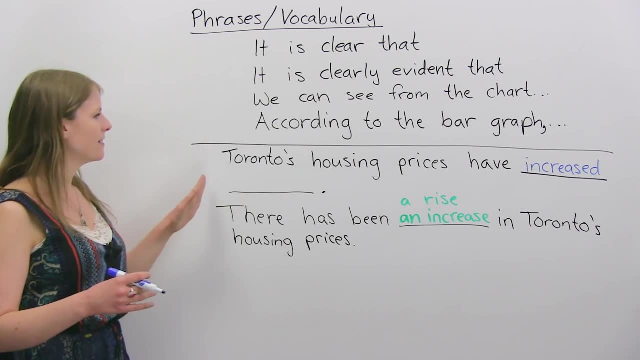 Okay, So it's good to know these, but use a couple of them and don't use them for each sentence, because you don't want it to have too much repetition. Okay, Another thing that will help you in terms of describing bar charts or bar graphs is 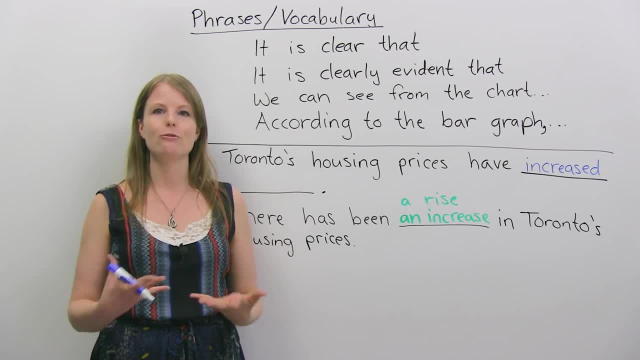 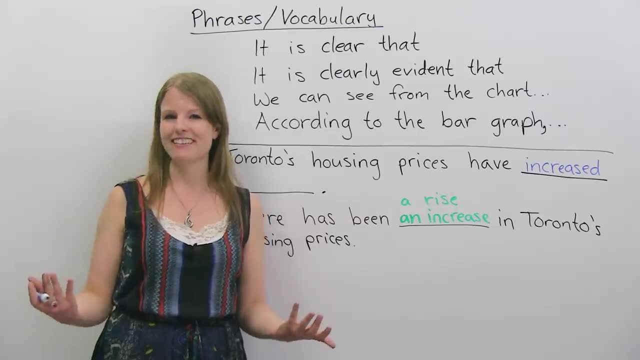 your vocabulary. It's very important that you have, You know, a high level of vocabulary. for the IELTS. You want to show that you know multiple words that have the same meaning, but that the words are different. So I'll give you an example. 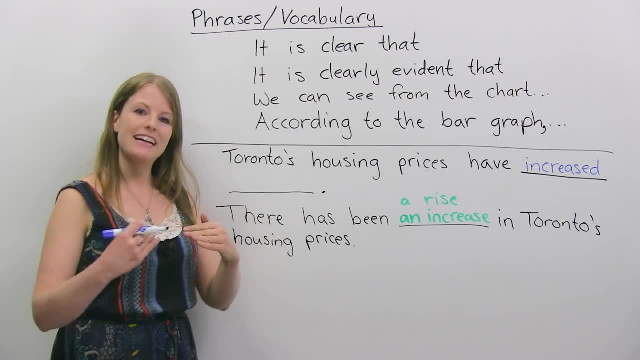 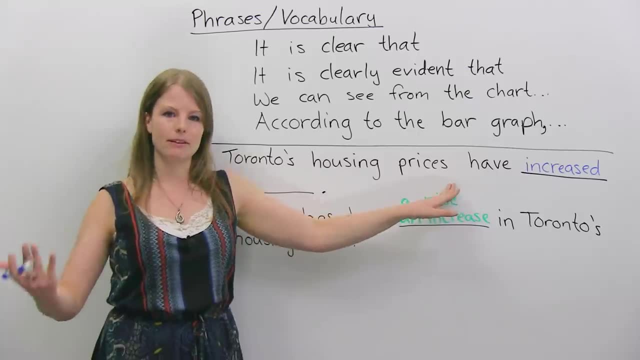 One thing we just talked about was housing prices and how there's been an increase. So I could say Toronto's housing prices have increased and you know, I'd probably give the amount at 5%. Now, this is great, But one problem students have is that they don't know how many houses they're going to have. 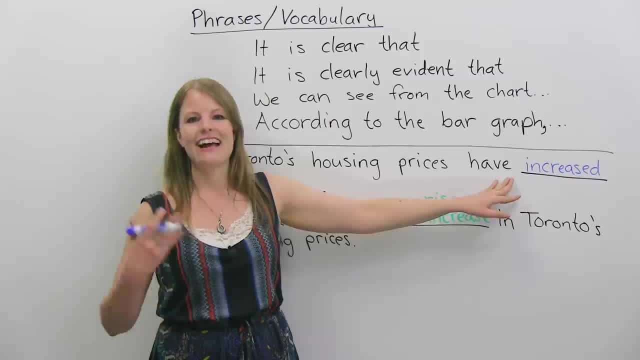 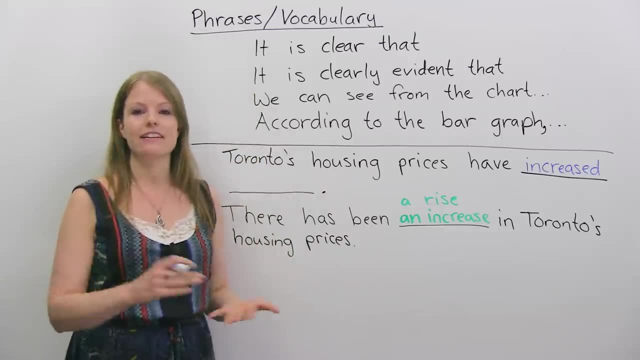 One problem students have is they keep using the same word again and again, and again, and so they don't get as high a score on their vocabulary. So we could add something to this to make it, you know, a bit more special or a bit. 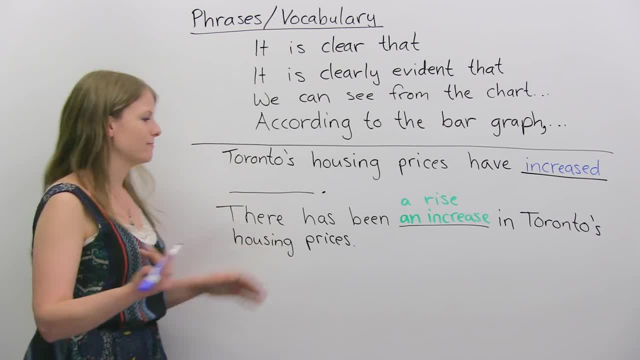 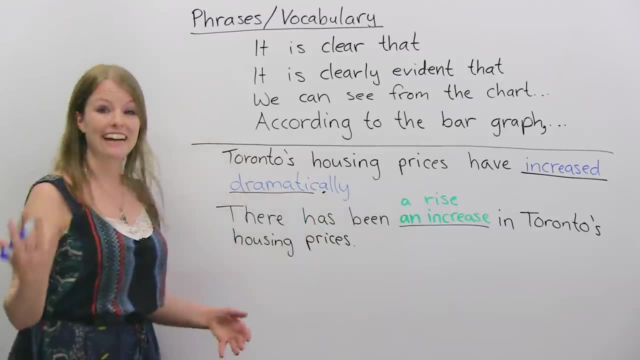 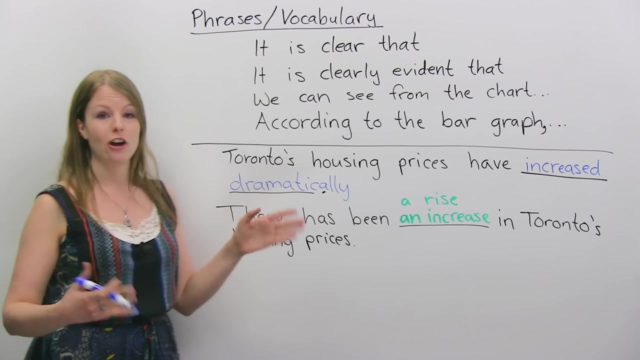 better. You know, maybe we can add an adverb. We have words like dramatically or steadily, So there's different things Slightly, which means just a little bit, So we can add an adverb here to describe what kind of increase was it? 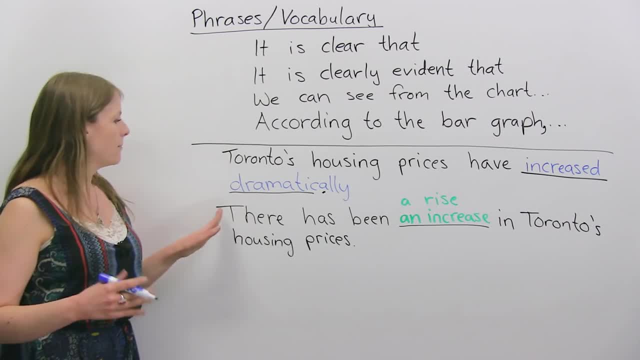 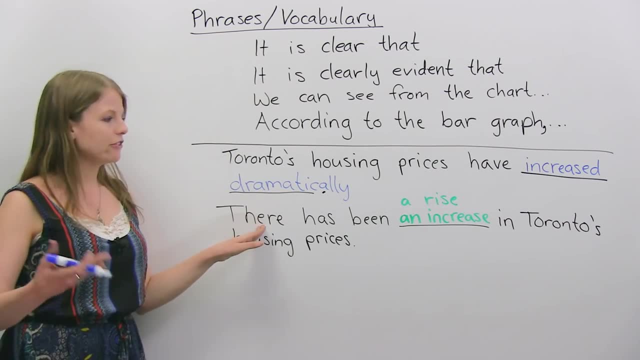 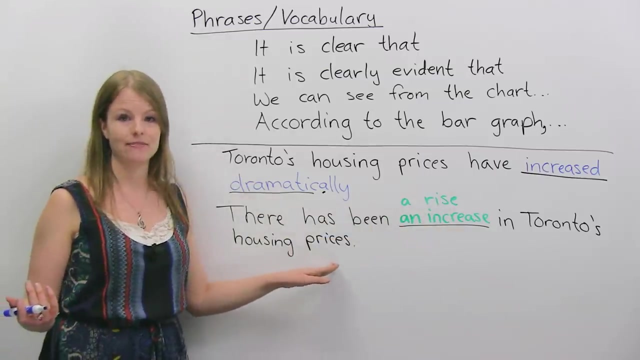 Was it a big increase or a small increase? We can also use increase as a noun. In this case it's a verb, but we can change this so it's in the noun form. now There has been an increase in Toronto's housing prices. 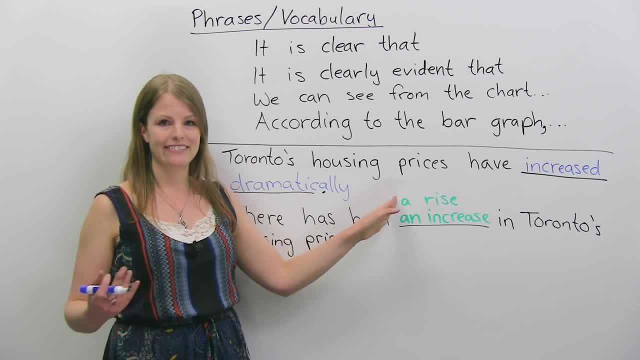 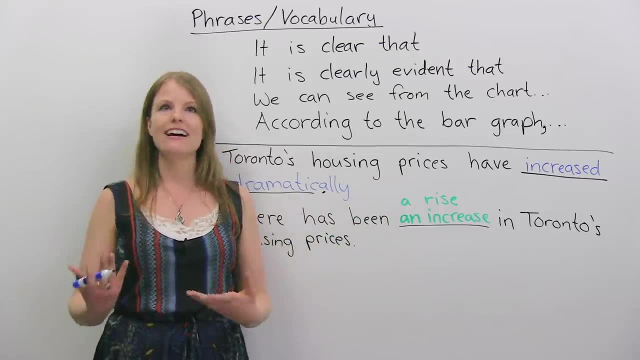 Or we can use a different word altogether. There has been a rise. A rise is a synonym of increase. They have the same meaning. They have the same meaning but they're different words. So finding synonyms that you know you'll often have to talk about increases and decreases. 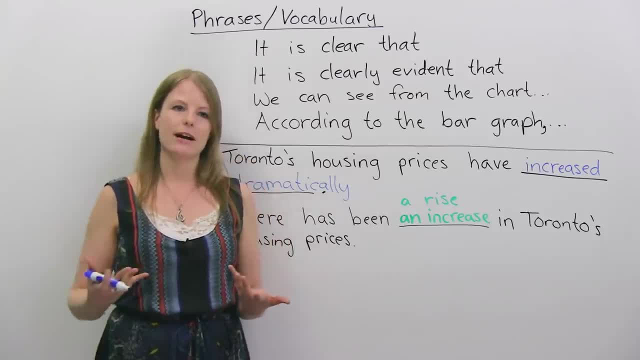 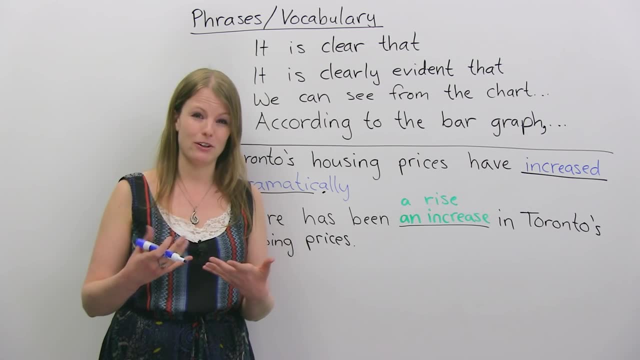 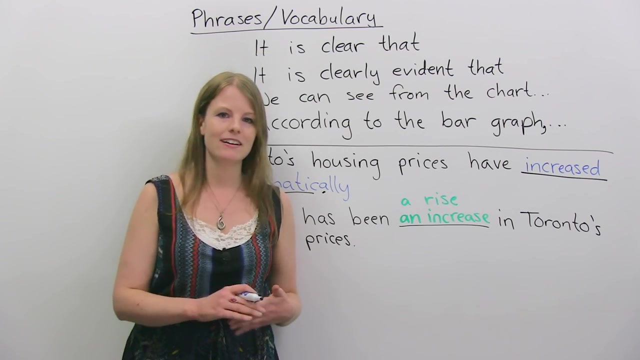 so finding And staying steady, So finding ways to you know to say these words, but to have multiple words that mean the same thing, synonyms of these words- is really, really a good idea in order to improve your vocabulary. mark on your writing for the IELTS. 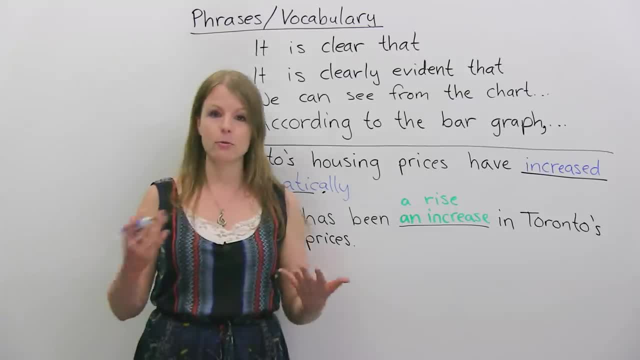 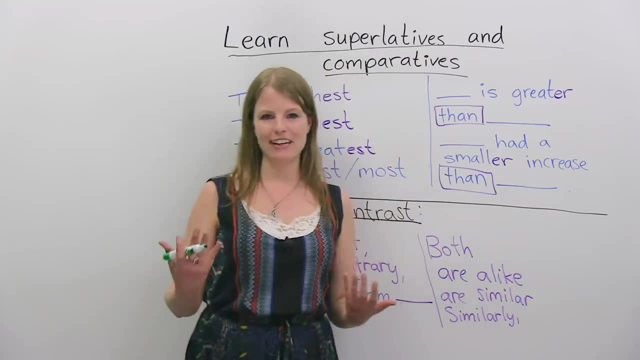 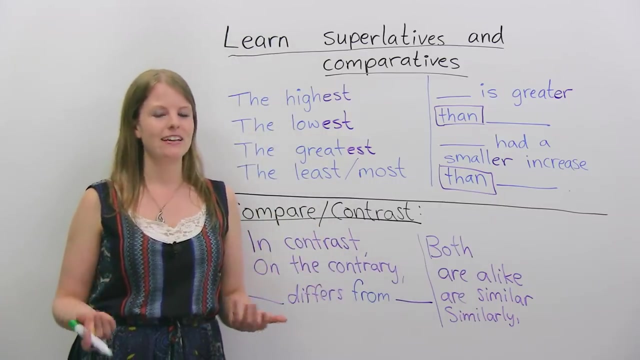 Okay So. So let's look at some more tips on how to improve. Okay, So I have two more tips on how to really help you with looking and analyzing bar charts or bar graphs. One of them is knowing your grammar. You get marked on the IELTS for how well you're able to write in terms of your grammar. 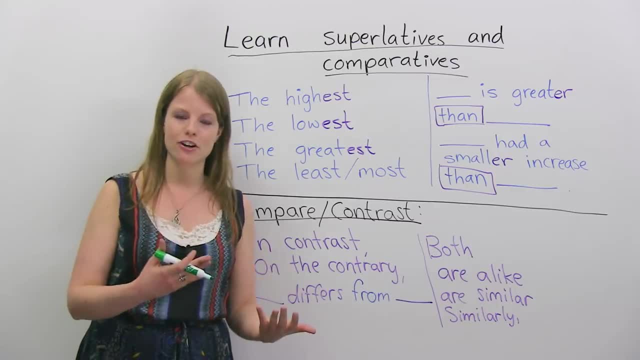 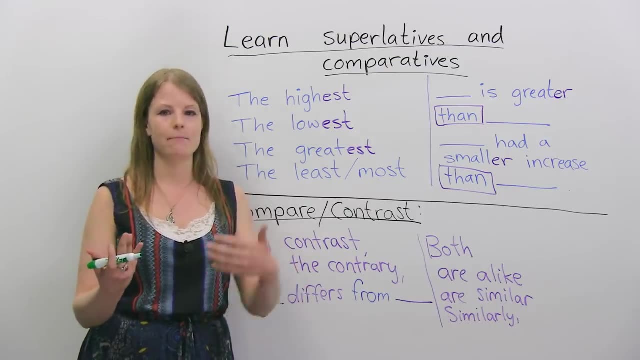 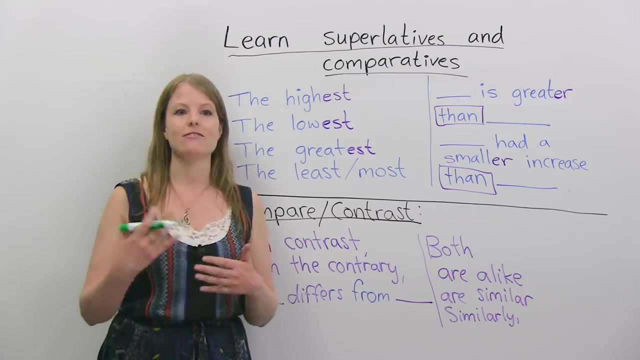 So, on this task, when you're looking at bar charts, you're often asked to compare different things. So in the case that we looked at before, you had to compare Vancouver to Toronto to Montreal, But you might be comparing different things. Maybe you're comparing, you know, hobbies of men to hobbies of women. 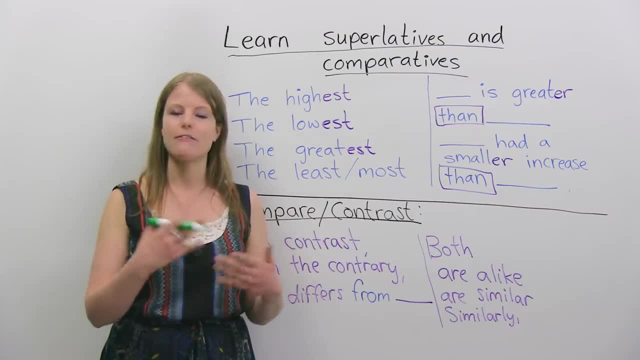 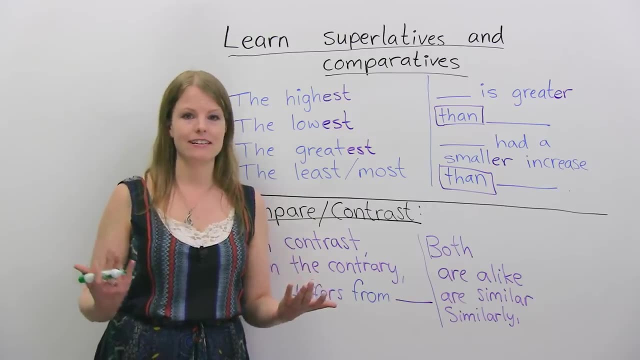 Or maybe you're looking at different ages and you know levels of schooling or something like that, So you'll probably have to compare and contrast different things. So one thing you should know is how to make superlatives Okay. So one thing you should know is how to make superlatives. 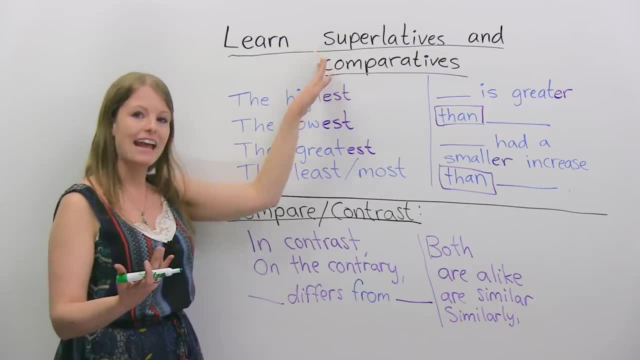 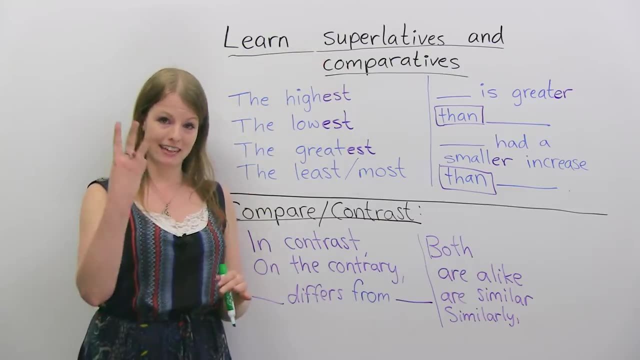 Okay. So one thing you should know is how to make superlatives Okay. Now let's look at superlative sentences and comparative sentences. So, as a reminder, superlatives is when you're comparing three things or more. You could be comparing three, four, five, six, ten. 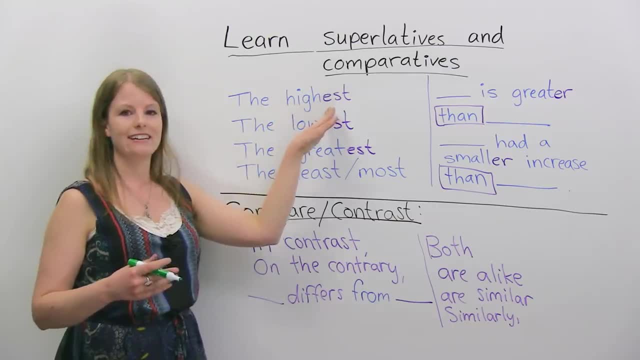 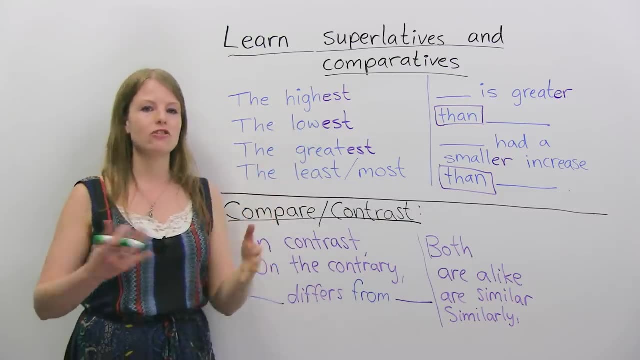 You use a superlative And what you're doing is you're saying: out of those three things, which is the highest, which is the lowest, which is the greatest? Pretty much you could do it with anything. for example, if you're looking at mountains. 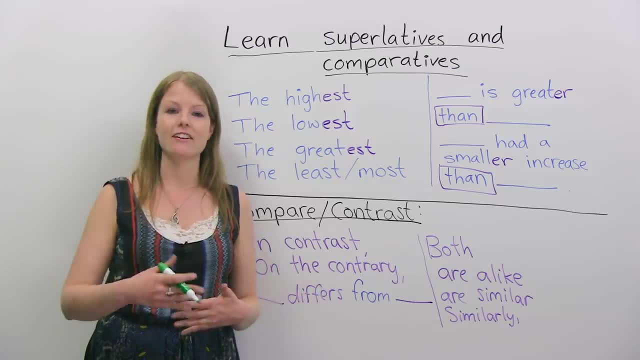 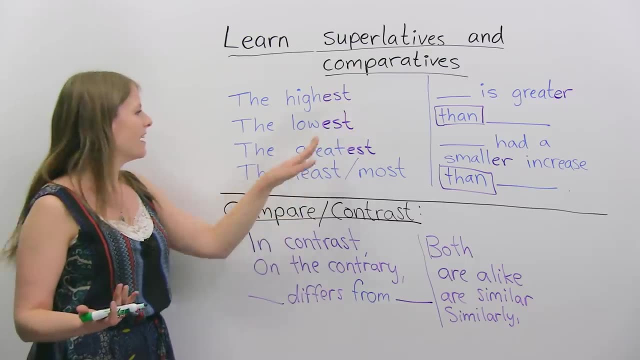 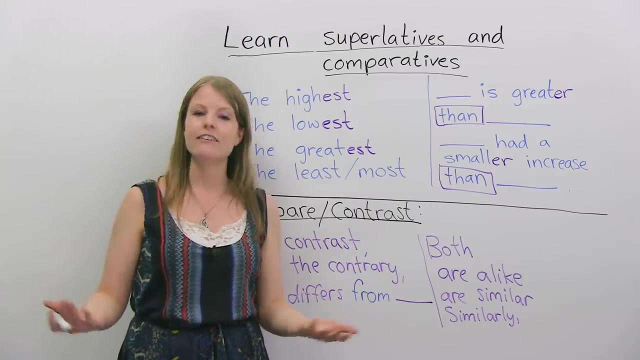 a superlative would be Mount Everest. Everest is the tallest mountain in the world, So superlatives have this ending "-est" and it also has the in front of it. Okay, So what we were talking about with housing prices: Vancouver has the highest housing. 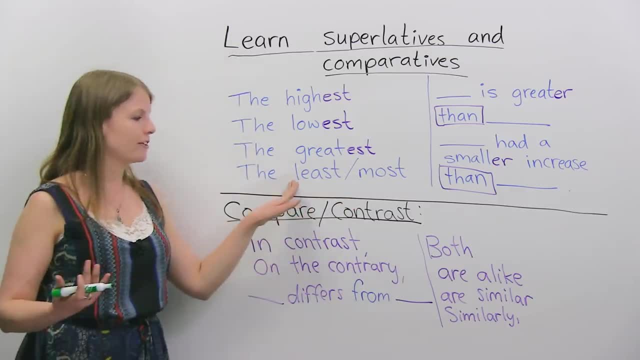 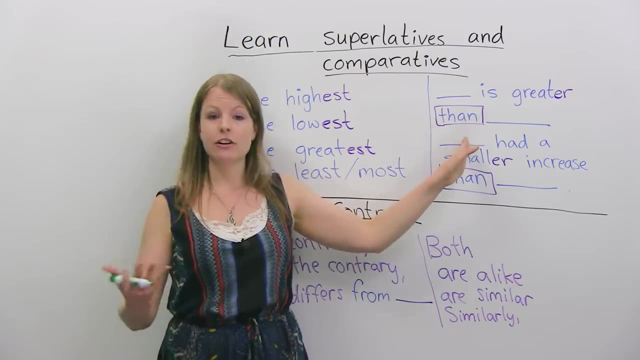 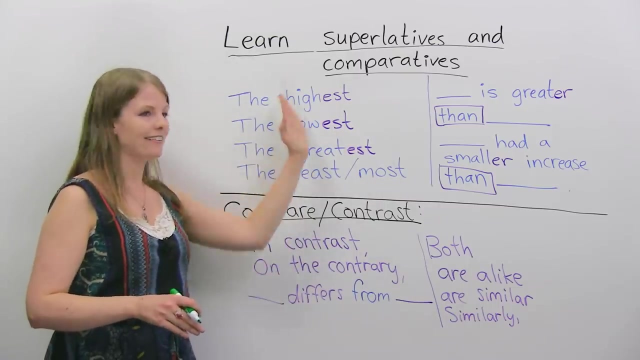 prices as an example. You also have here the least and the most. These are also superlatives. Then we have these things called comparatives. We use comparatives when we're comparing two things. So superlatives, this is for three or more. 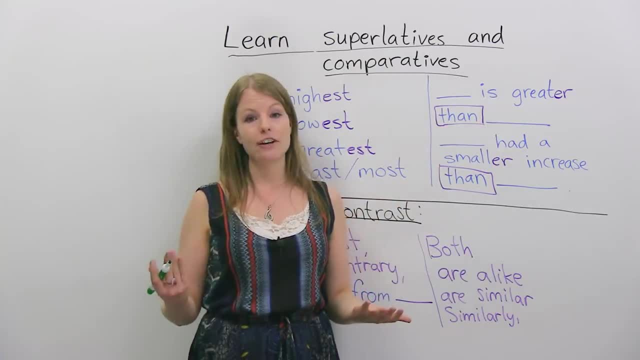 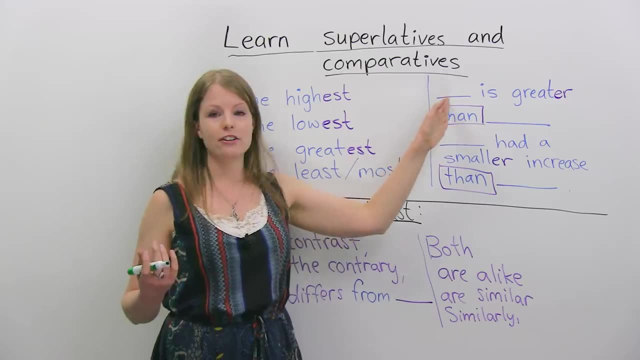 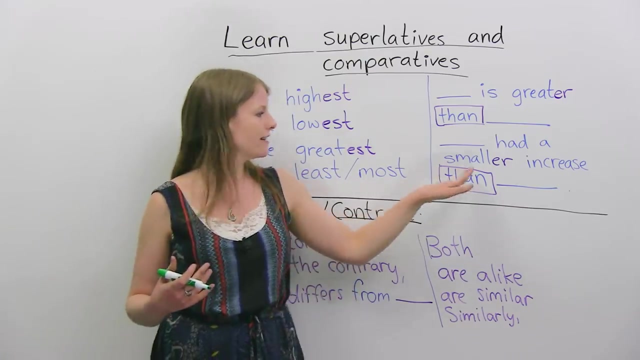 Comparatives are when you're just comparing two different things. So, for example, if we wanted to compare Montreal and Toronto, we could say Toronto has a higher population than Montreal. Or you know, with housing prices, Montreal had a smaller increase than Toronto. 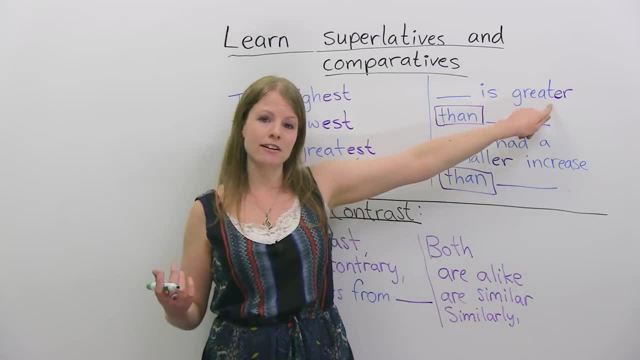 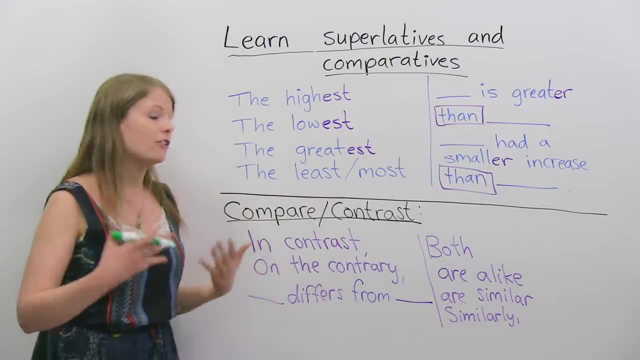 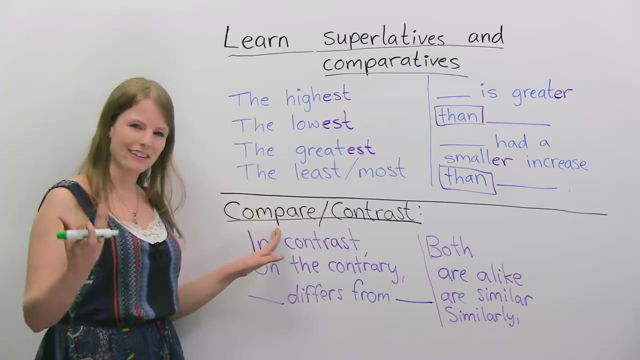 Okay, So the key here is you have "-er" and you also have "-van", So these are comparatives. Another thing that you can really do to help your mark on the IELTS and your vocabulary is using different transition words for compare and contrast. 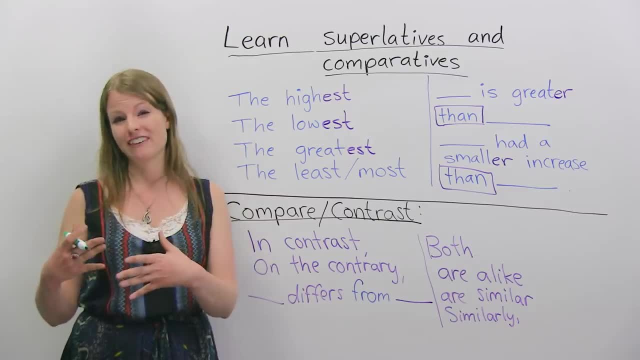 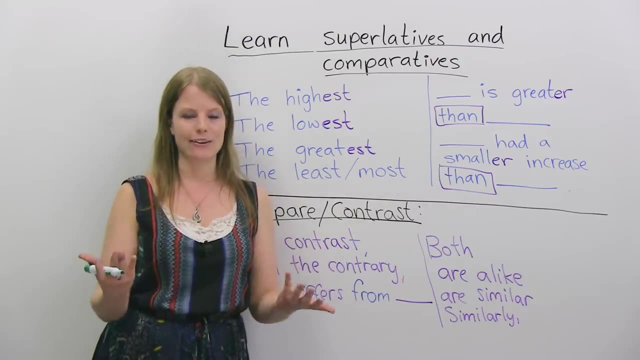 Compare is where you're saying how do I compare? You're saying how things are the same or similar. Contrast is when you're saying how things are different. So on the IELTS Task 1, you're going to have to say how things are similar and how things. 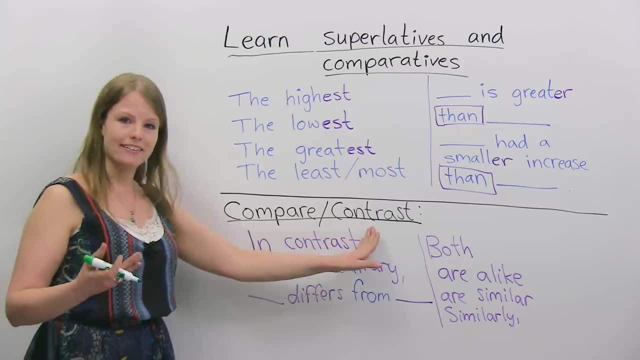 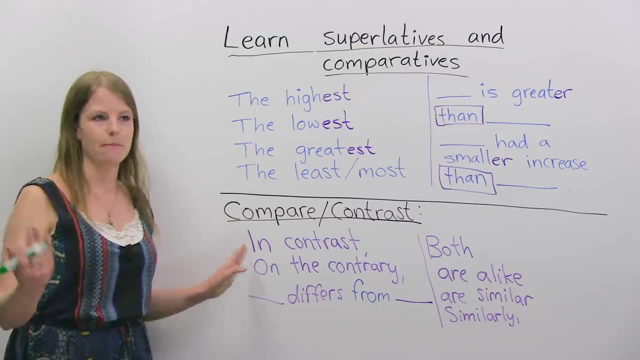 are different. So, in terms of contrast- we have some great examples of expressions here- You can use the words in contrast. So, for example, Vancouver has very high housing prices. In contrast, you can use the words in contrast. 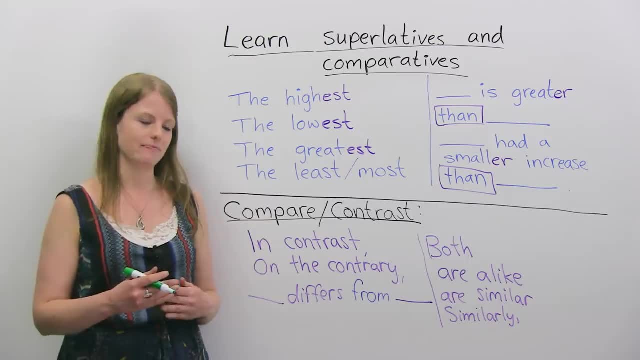 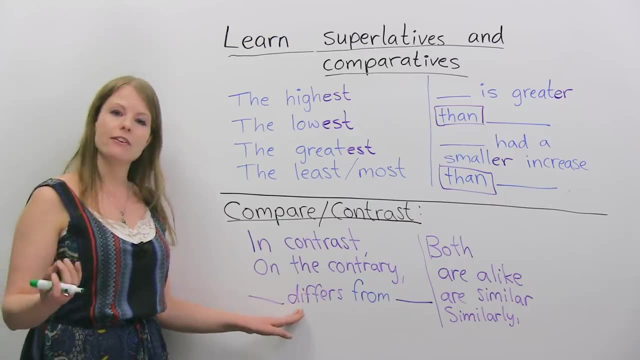 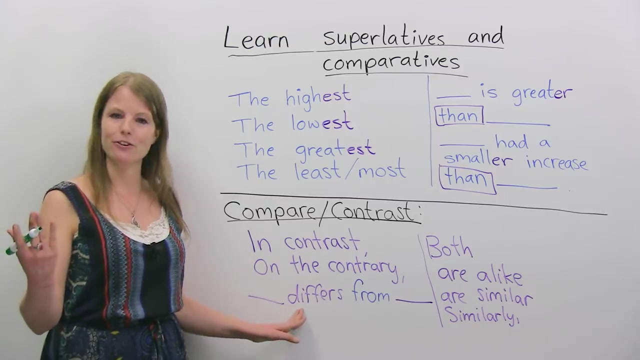 In contrast, Montreal has low housing prices. You can use the words on the contrary in the same way as in contrast. You can also use the verb form of different. A lot of students don't know about this word, but I think it's great whenever you're doing. 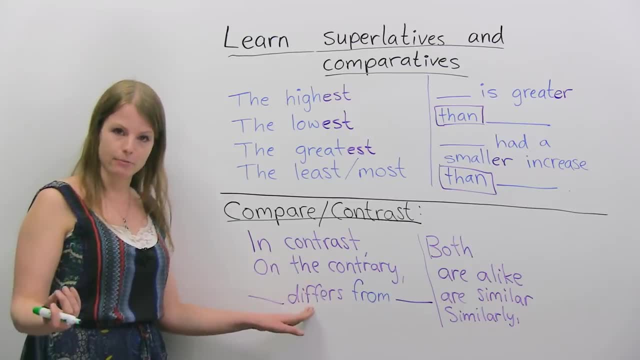 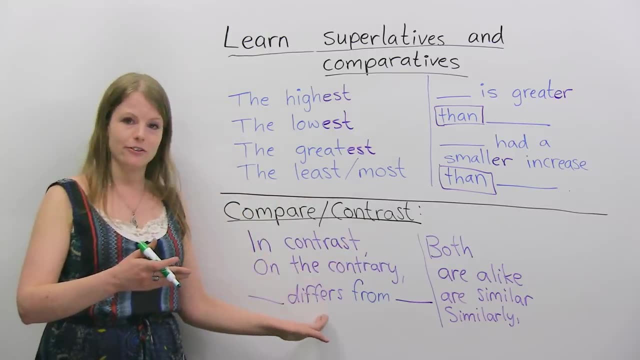 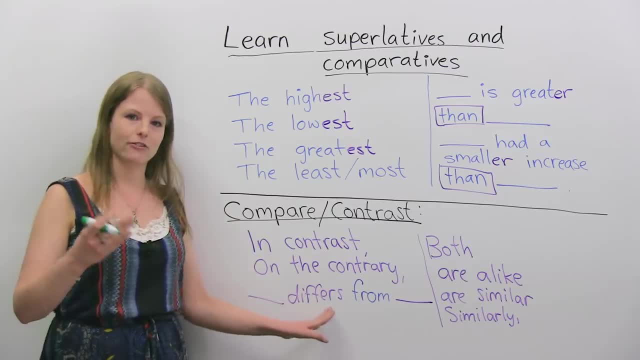 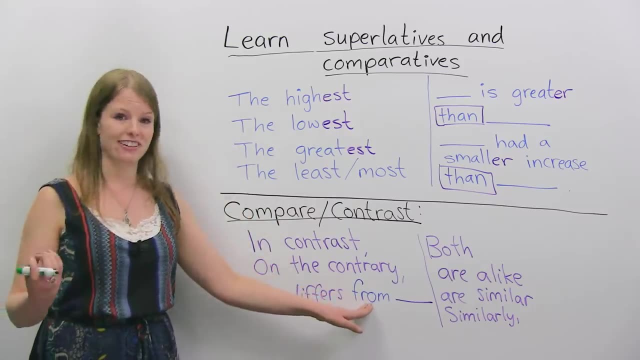 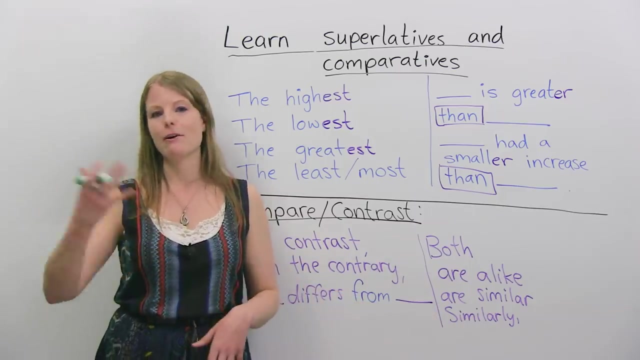 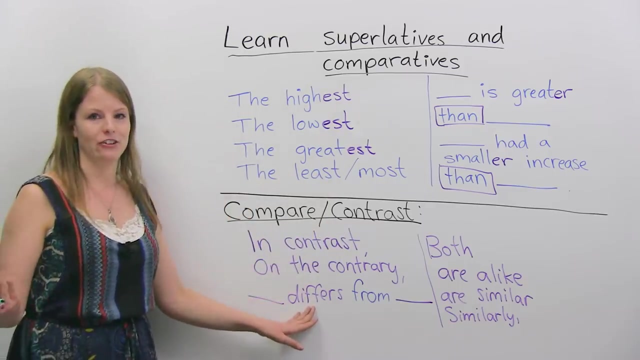 Montreal differs from Toronto. It just means that there's a difference. Notice also the preposition that comes after differs. We say differs from something. If I wanted to talk about apples and oranges, apples differ from oranges. Okay, So very good vocabulary here to use. 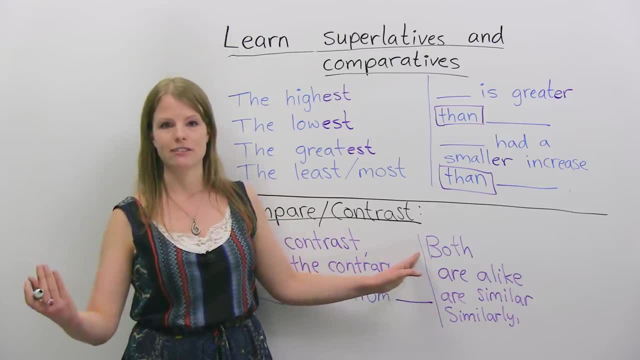 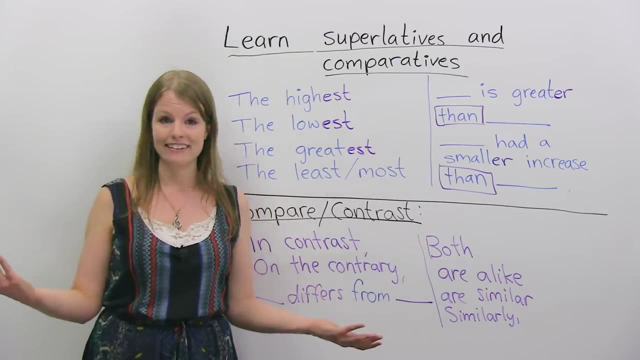 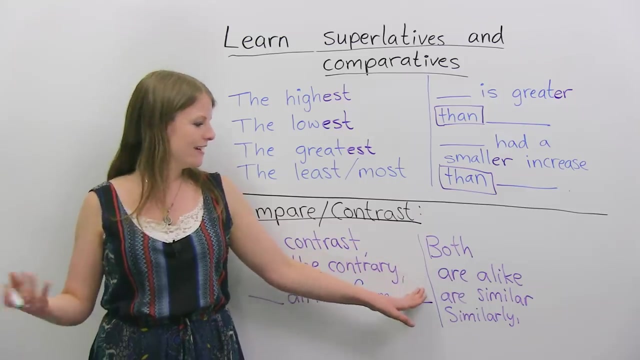 We also have words for when we're talking about how things are similar, When we're comparing things. So we have the word both. Both Toronto and Vancouver are great cities. Toronto and Montreal- Montreal, sorry- are alike in many ways. 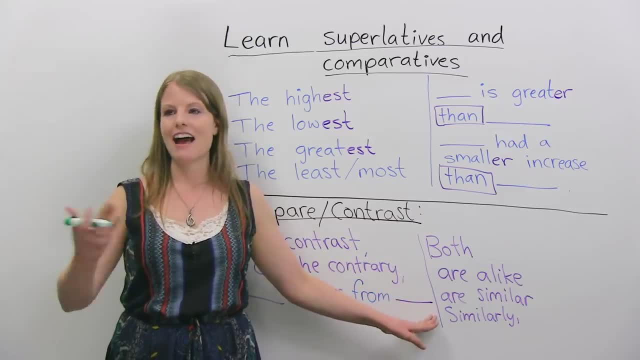 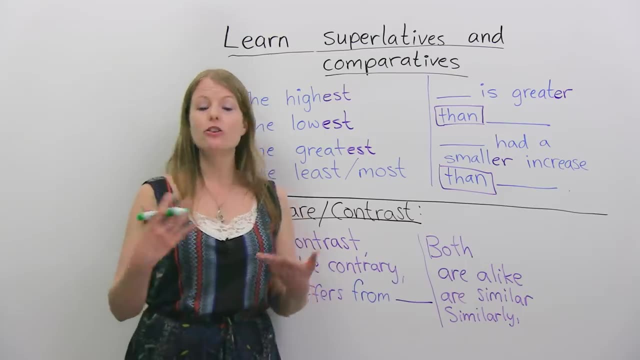 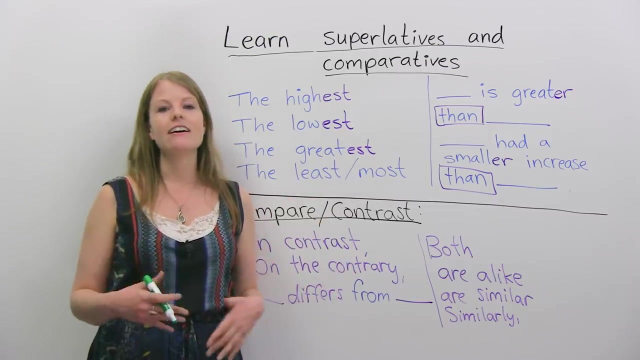 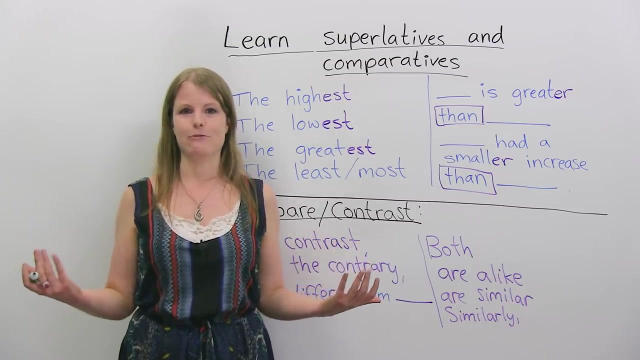 They are similar. Toronto has had an increase in housing prices. Similarly, Vancouver has had an increase. Okay, So using these types of words can really help you in your mark in terms of your vocabulary and organization. So we've covered a lot today and you might be asking questions like: oh my God, comparatives. 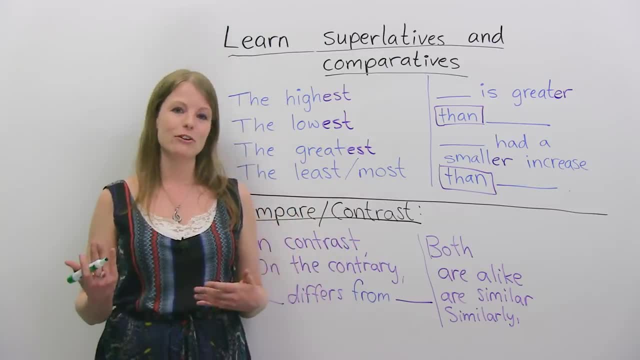 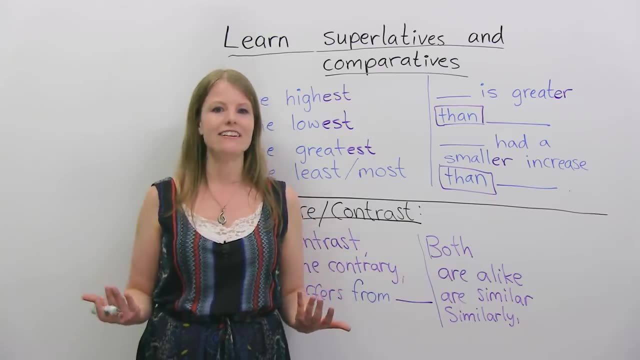 superlatives? ugh, I don't remember any of that, Or you might be confused by it. Similarly, with compare and contrast, you might think: well, how do I use this in a sentence? Those are all very good questions, and I wanted to tell you we have a lot of resources that 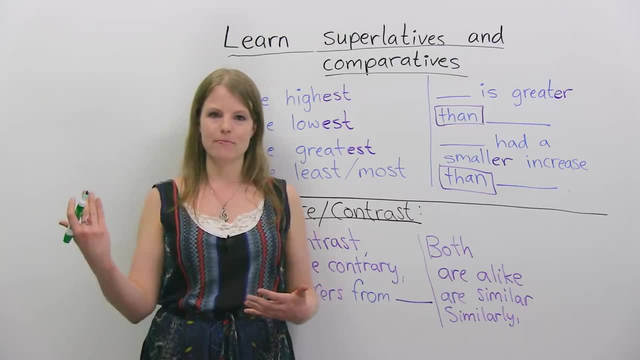 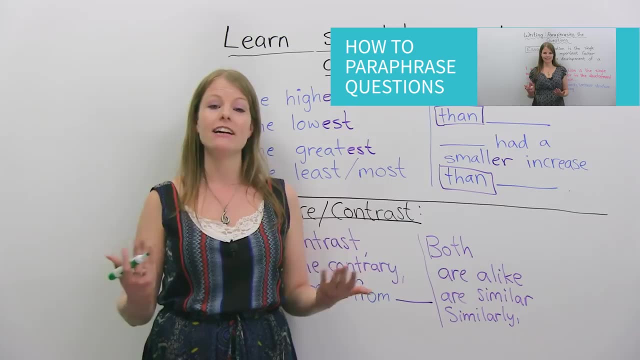 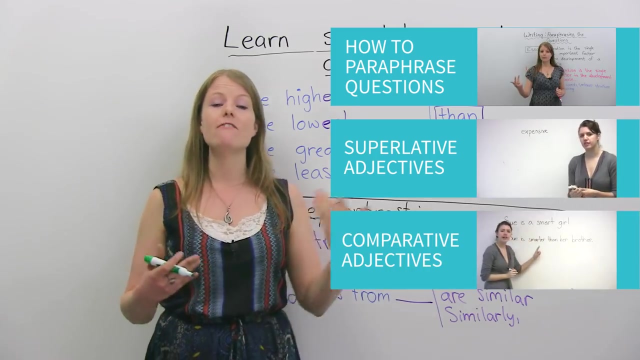 can help you with that. So earlier in the video I talked about how you want to change the question into your own words. We have a video on how to do that. about paraphrasing, When I talked about superlatives and comparatives, we have a video on that, on what they are. 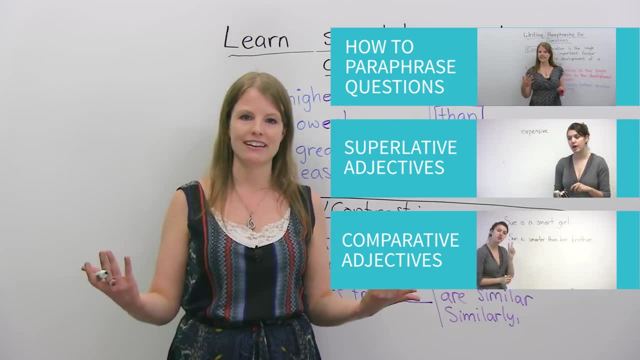 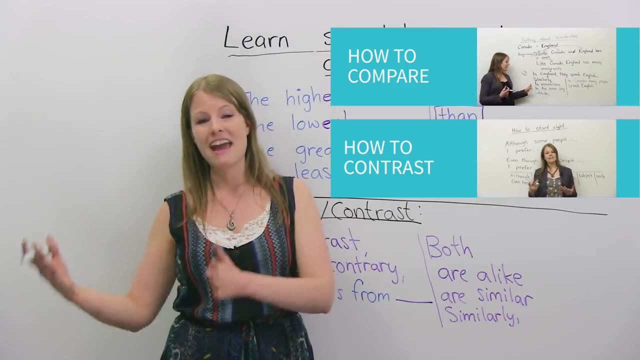 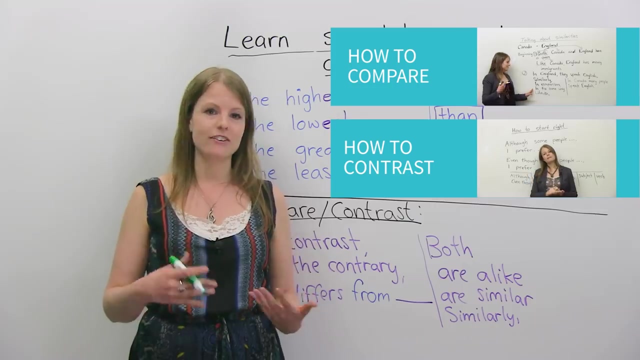 and how do we, How do we write them, How do we do them correctly? Compare and contrast. We have a great video on some expressions we can use when we compare and some expressions we use when we contrast, So these extra videos are really good for this task, so I highly recommend watching. 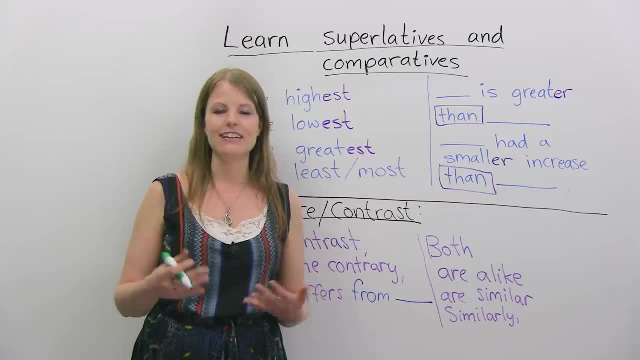 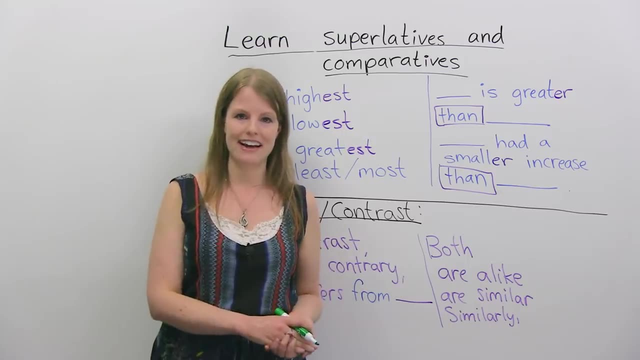 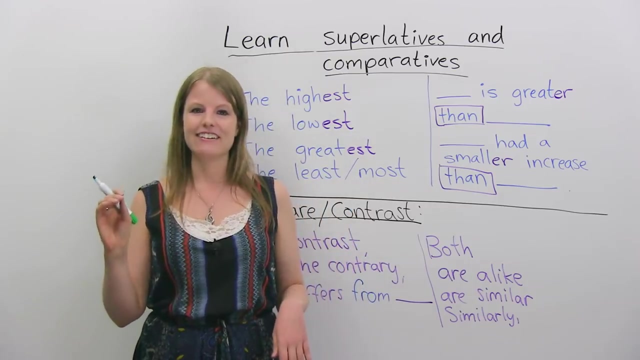 them and really understanding how these things work. So we've covered a lot today and there's a lot more that you can study, so I invite you to check out our website at www. Ugh sorry, wwwengvidcom. 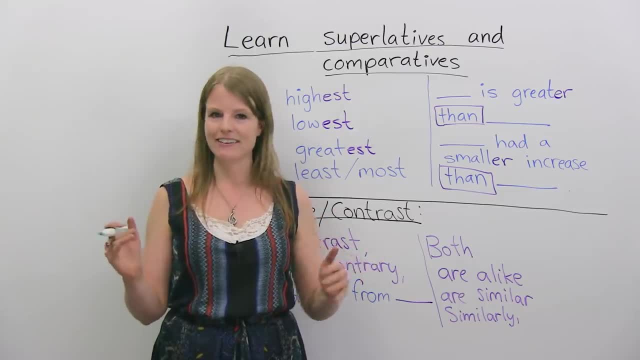 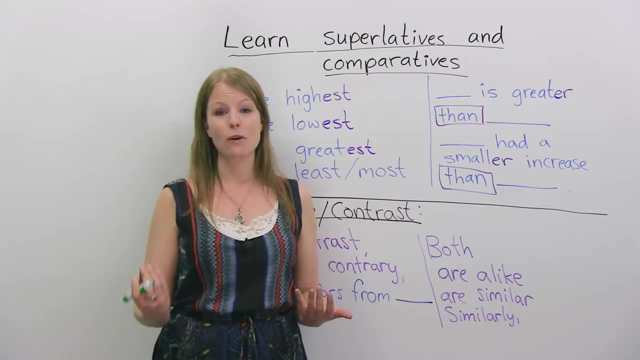 There you can actually find more resources on all sorts of different things, I'm sorry, From IELTS to pronunciation to vocabulary, all sorts of great videos, And you can also try our quiz on bar graphs, which can really help you practice everything.